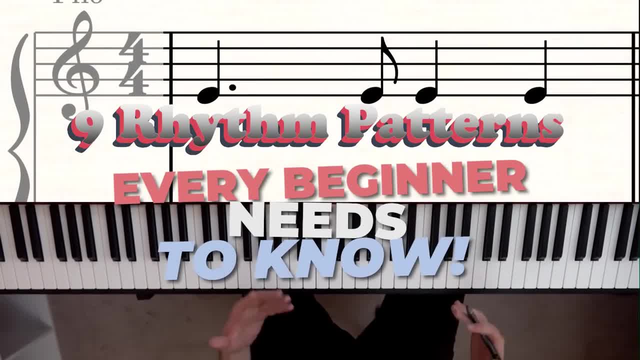 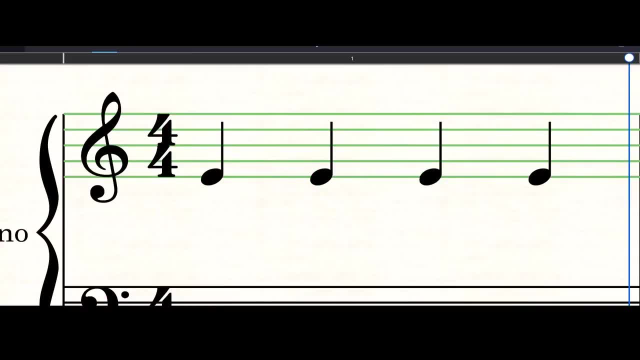 There are nine rhythm patterns every beginner needs to know to play piano effectively. but to explain any of them I first have to explain the concept of subdivision. So here we have a measure of four, four, four quarter notes. very simple: count it as one, two, three, four and then. 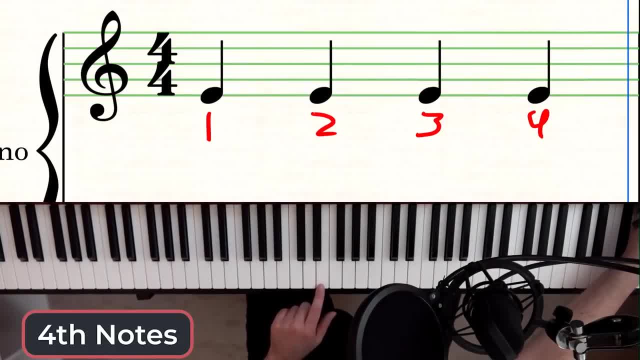 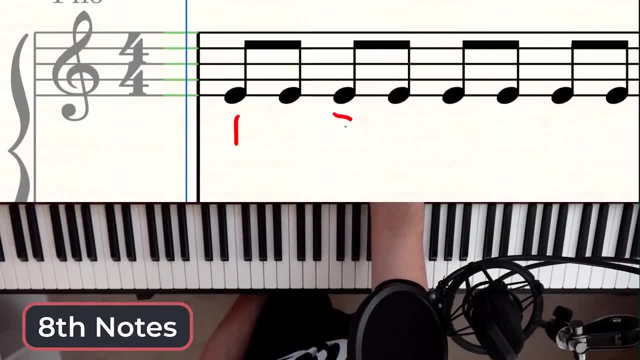 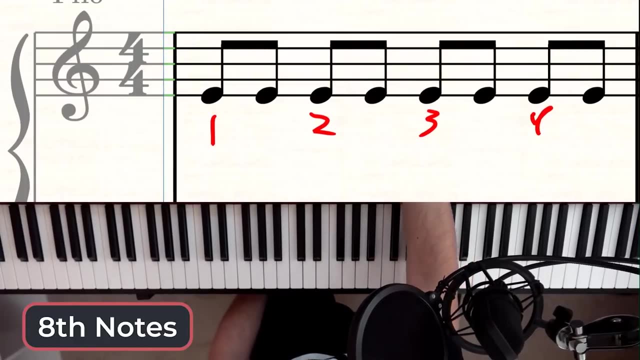 on the piano. of course that's just going to be one, two, three, four, and now we're actually going to get into subdivision. So now we still have our four beats here. they're right here: one, two, three, four. but because an eighth note only gets half of a beat, we now have to basically fit two. 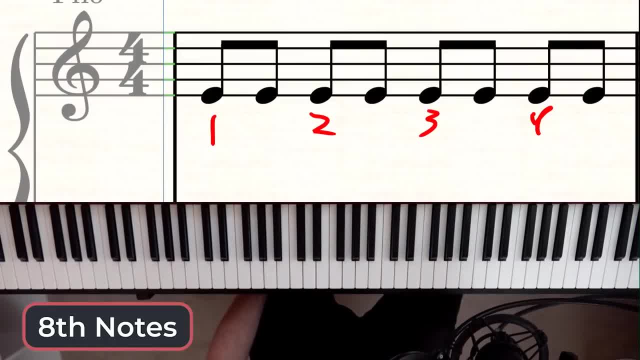 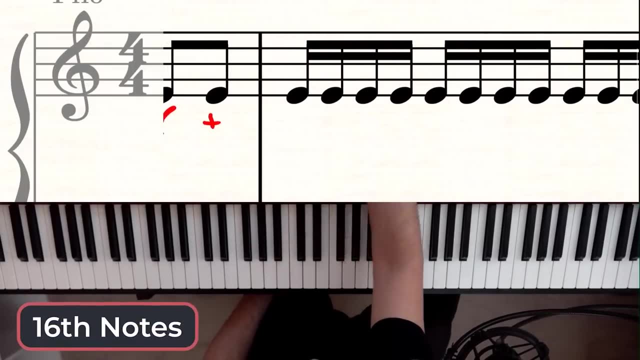 notes in every beat and we use the term and it looks like a plus sign. So now, instead of one, two, three, four, we're going to be counted one and two and three and four, and I still had my quarter notes counting out with my finger and then hitting the eighth notes like that. Now we're going to 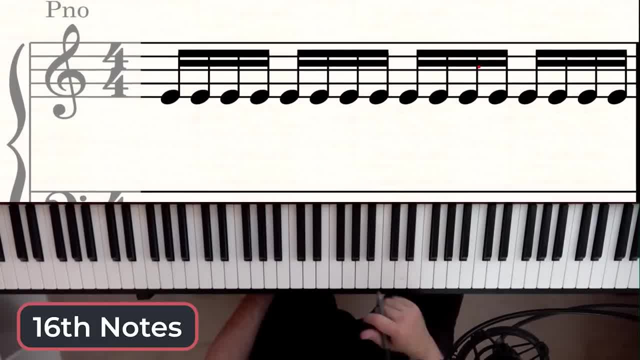 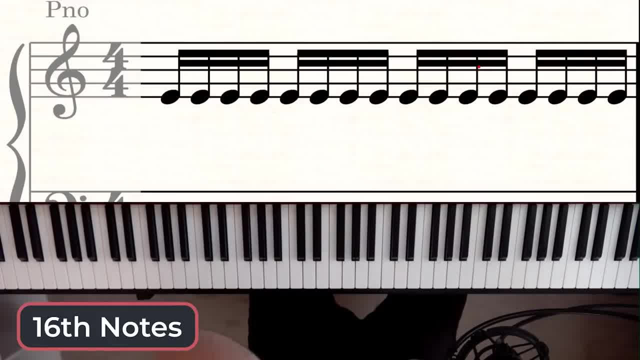 going to split it down even further to 16, and then we're going to split it down even further to 16 note subdivisions and I'm going to explain when you might use 16th or eighth note subdivisions in note subdivisions in your piece. but here we're breaking down each beat into four, four equal parts. 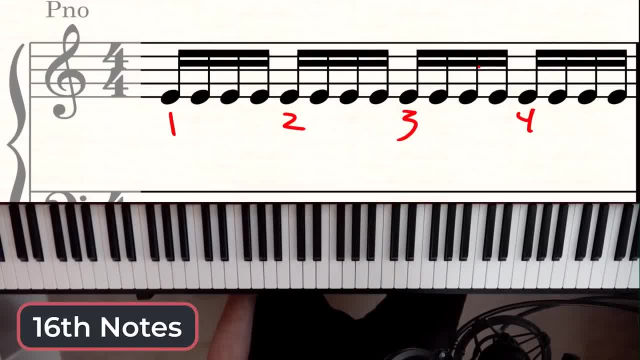 so we still have our beats one, two, three, four, and we even still have the second half of each beat here, the ands. so one and two, and three and four, and just like that. so now we have to account for our missing notes, because now we're splitting each of those. 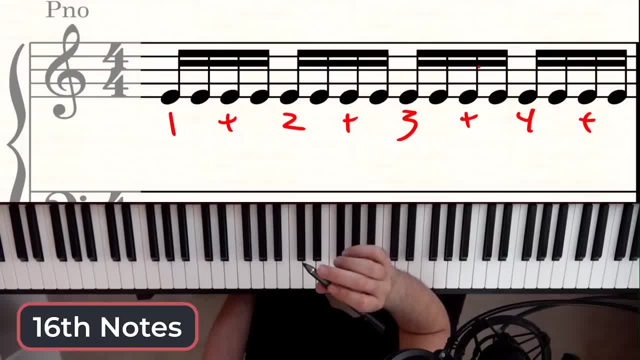 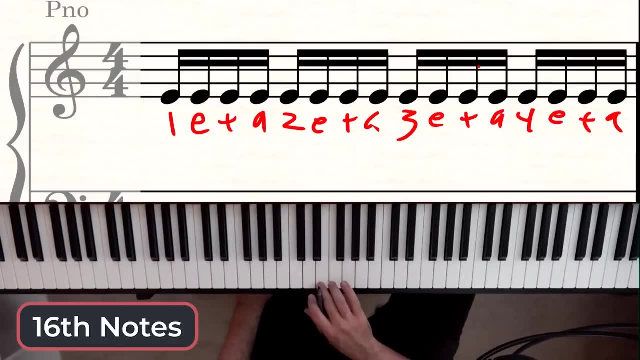 into halves and we use this following terms: so we have 1 E and uh, 2 E and uh, 3 E and uh, 4 E and uh. so instead of 1 and 2 and 3 and 4, and it's now 1 E and 2 E and 3 E and uh, 4 E and uh. 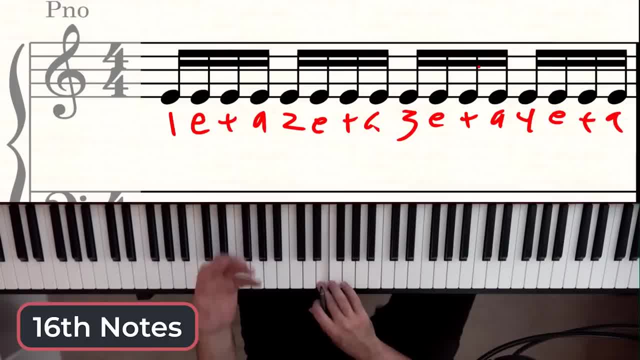 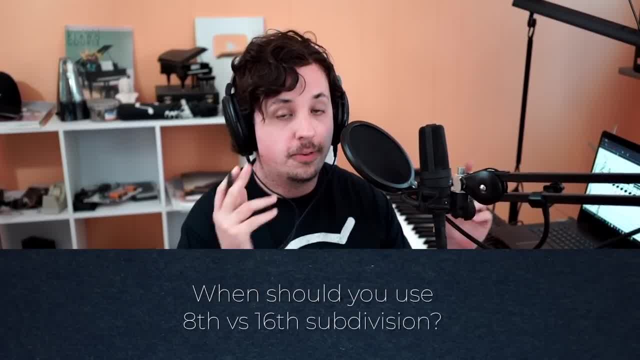 you still have to keep up with the beats of 1, 2, 3, 4, but now you're just putting in 4. instead of three. So when should you use 16th note subdivision versus eighth note subdivision? Well, here it is. 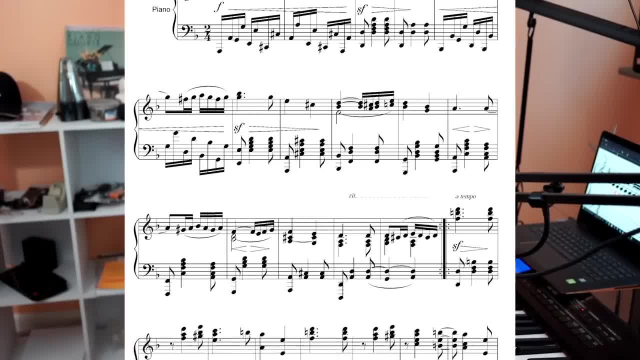 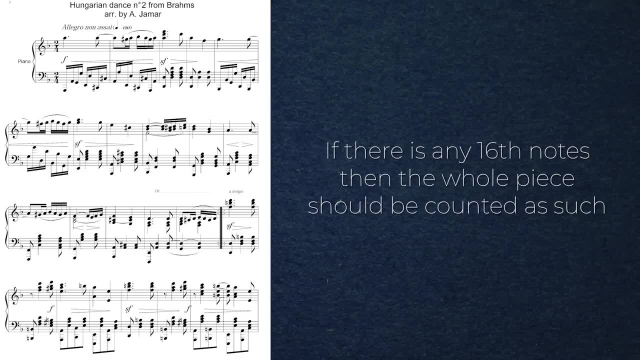 Here's the answer. Everybody asks me this: If you have any 16th notes in your song at all, it can be a 16th rest somewhere in the middle. You have to subdivide 16ths the entire time, even if you have quarter notes. 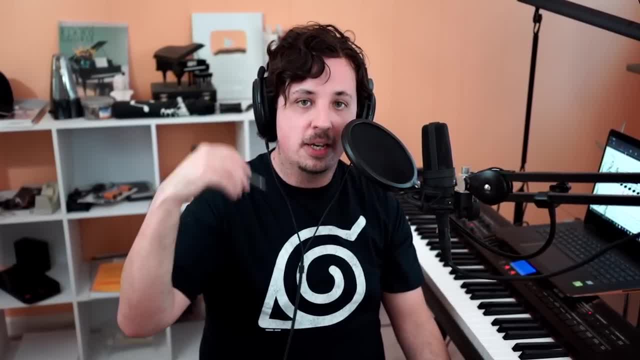 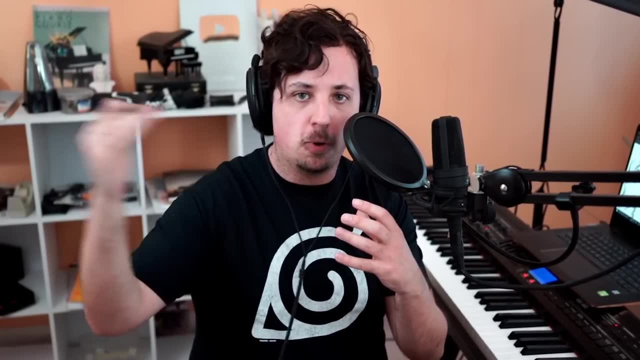 because what that'll do is that'll make sure that you are playing consistently throughout the whole thing And then, when you finally get to that measure of a 16ths, it's not gonna be so jarring to move from just counting flat quarter notes to 16ths and back. 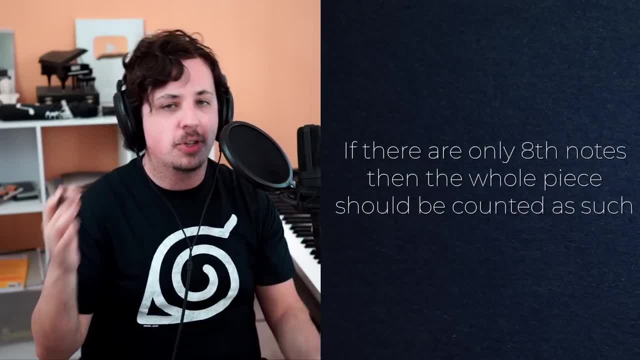 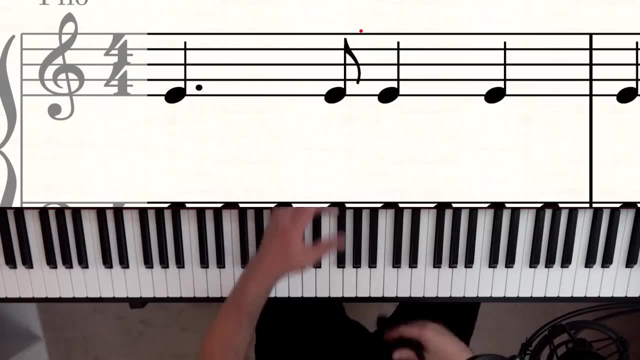 If you don't have any 16ths in your music, maybe just eighth notes, you can probably get away with just using the eighth note subdivision. Speaking of eighth note subdivision, here we have the rhythm I showed you right in the beginning, the dotted quarter eighth rhythm, which is these two guys. 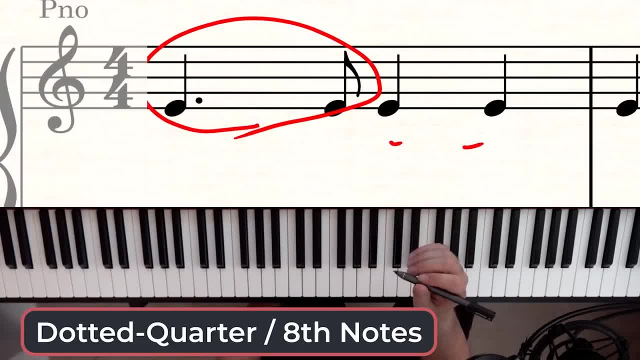 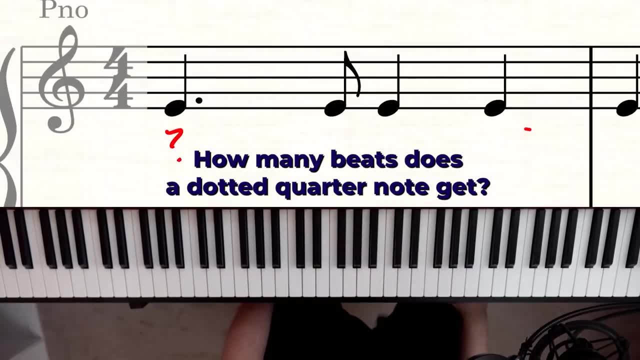 And then I just added in some quarter notes to fill out the measure. Now let me show you how you're gonna count this. So the first question I have for you is: how many beats does a dotted quarter note get? And you probably may know that it gets one and a half beats. 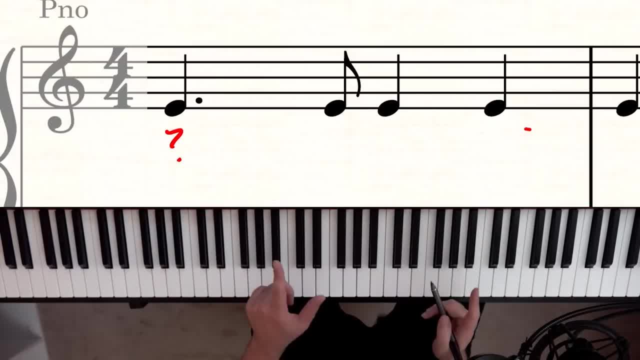 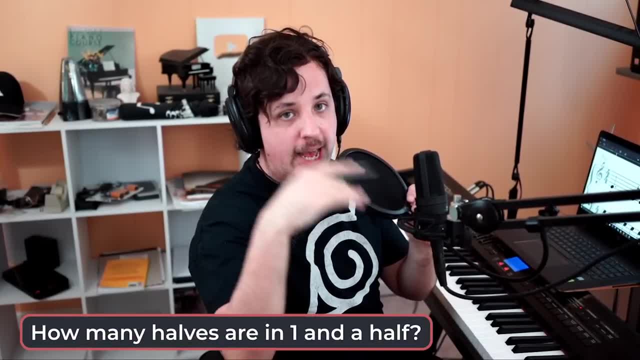 So how do we count that? Well, we use our eighth note subdivision as our friend. I have another question for you. How many halves it gets? one and a half beats right in the dotted quarter. How many halves are in one and a half? 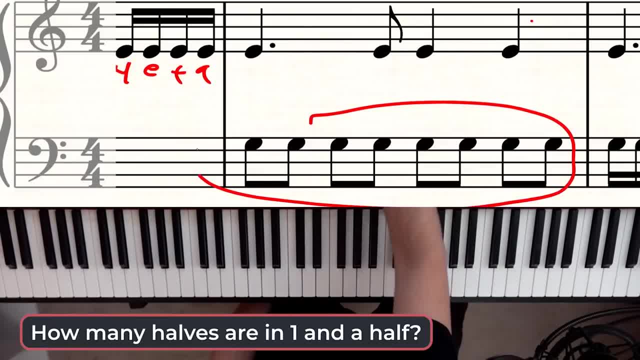 So to answer this question, I drew our eighth note subdivisions down on the bass clef so we can compare them. And the answer to that question is three right, Three halves of one and a half. because you have a half, you have another half. 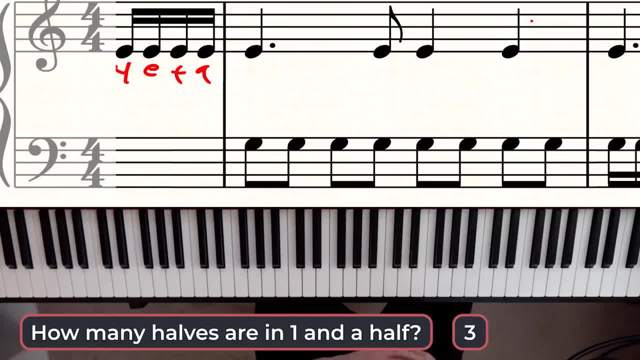 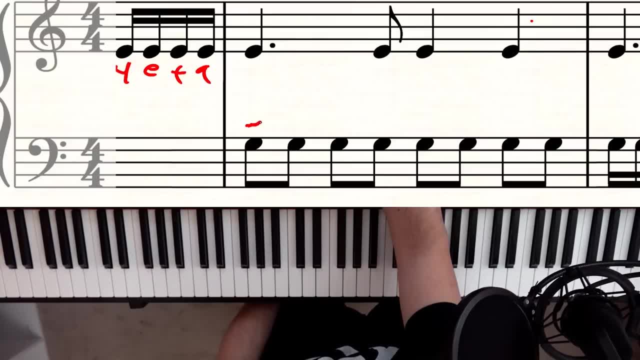 another half makes a whole, and then another half to make one and a half. And remember that each eighth note only took up half of a beat. So this dotted quarter note is gonna take up this eighth note, cause that's half of a beat. 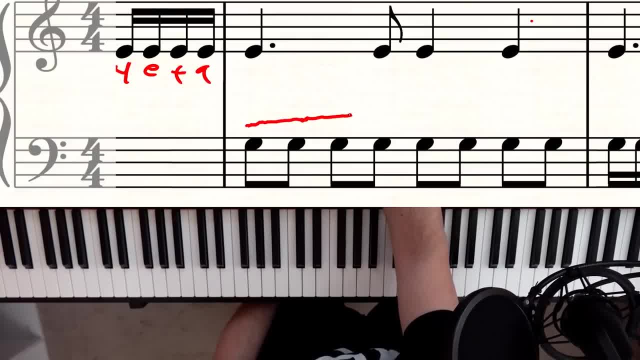 It's gonna take up this eighth note. that's another half of the beat. And it's actually gonna take up this eighth note. that's another half of the beat. So this is gonna be counted as one and two, and then you're moving again on the and of two. 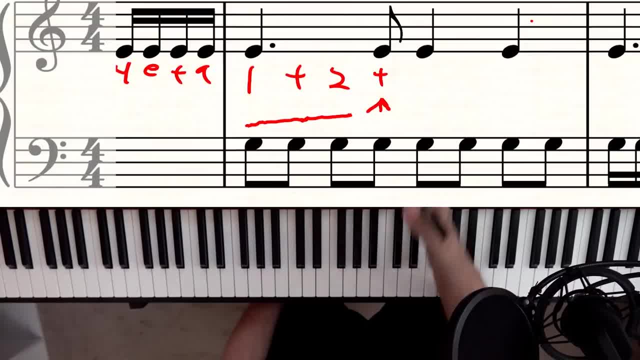 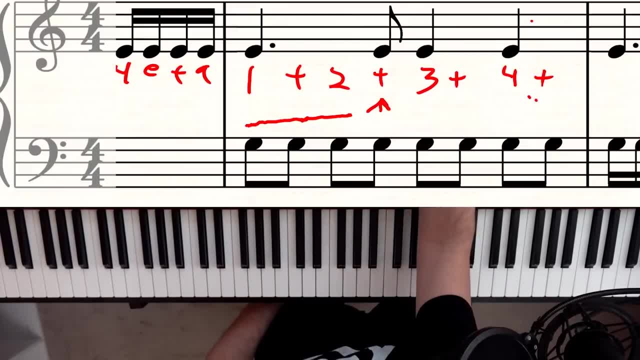 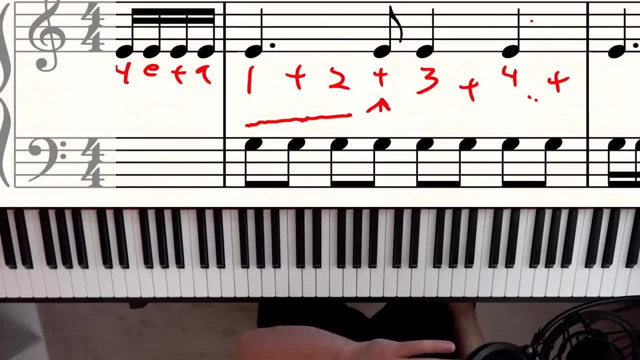 So one and two, and, and then, of course, you would count three, four, or would I? Well, no, you wanna be counting out your eighth note subdivision here? I should actually move these over so they're lined up, because that will help you count more accurately. 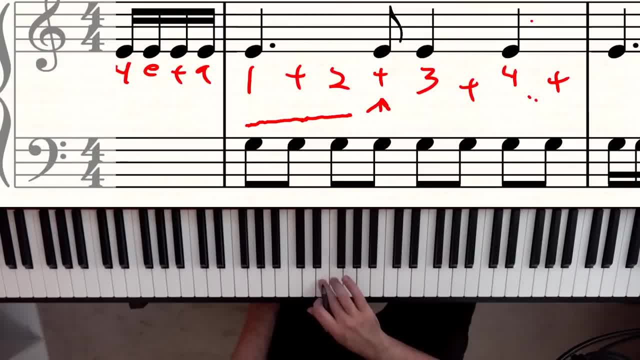 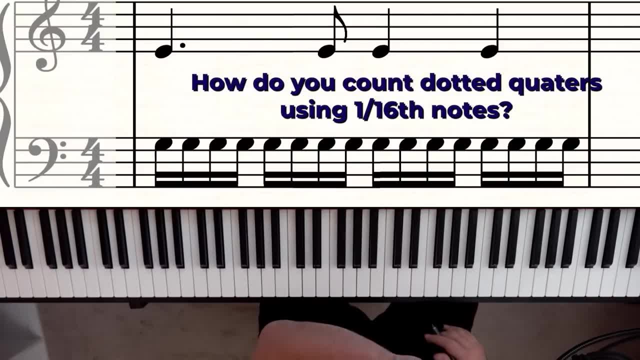 and consistently So. this rhythm is one and two and three and four, and So question: how do you count dotted quarters using 16th notes? Well, quite simple, Okay. so remember we said a dotted quarter gets one and a half beats. 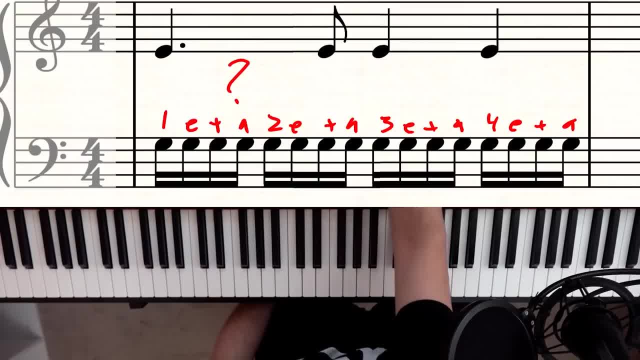 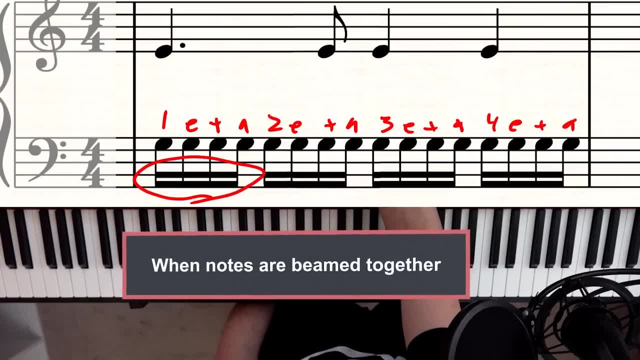 Well, how many of these is it gonna take up? Well, I have a tip for you. It's the best tip of the whole lesson. I'm serious. When notes are beamed together, that means they equal one beat. So we know that it's gonna take up at least one E and a. 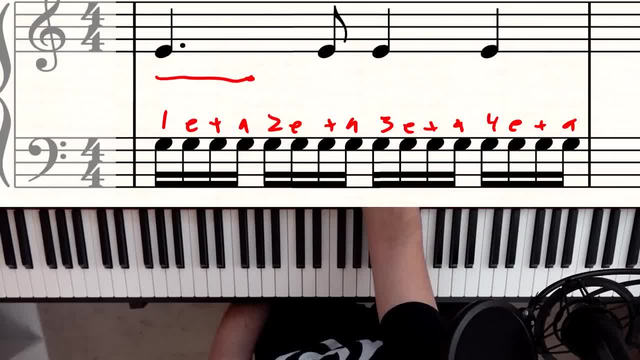 right, cause that's one beat, but we need half of a beat left, So that would be two E as well, because this would be the other second half of two, which makes sense, cause that's where the eighth note is. So it would be counted one E and a half. 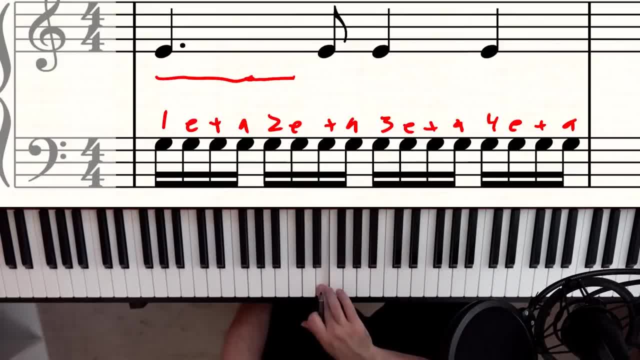 So it would be counted one E and a half. So it would be counted one E and a half, One E and a half, Two E and a half, Three E and a half, Four E and a half, Three E and a half. 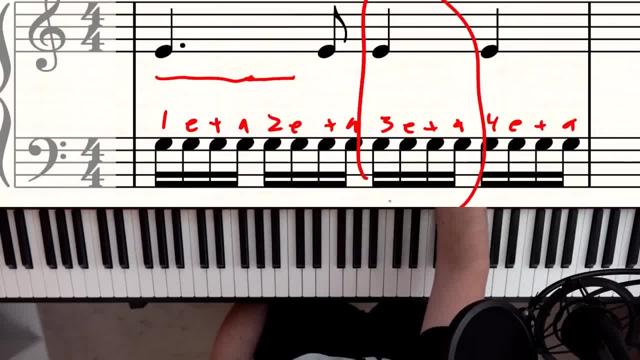 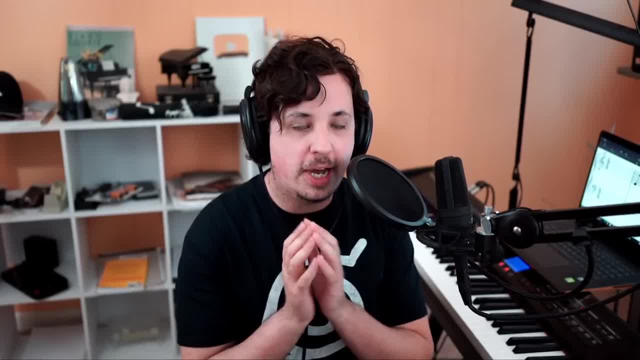 Four E and a half, Three E and a half. Remembering that you still wanna subdivide this beat and this beat, Why? Well, so you can count more accurately. There's an alternative way to count: that dotted quarter eighth rhythm, and we're gonna use pineapples. 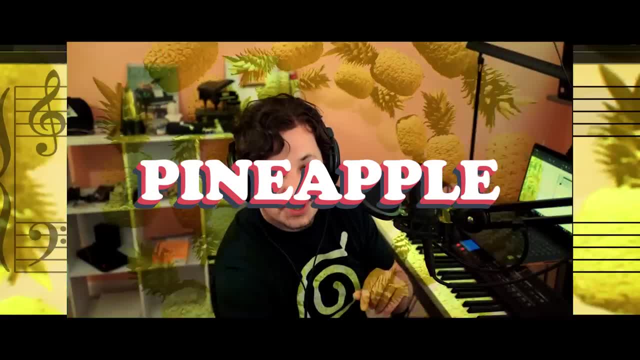 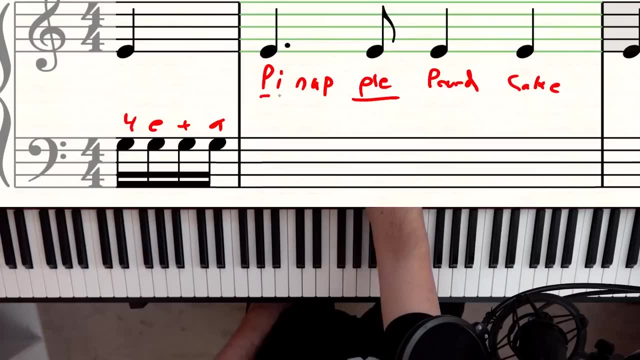 Yes, really. So we're gonna use the word pineapple, And let me show you actually how we're gonna do this. You can actually count rhythms by associating certain words with them and certain syllables within the word, So you can use pineapple with the dotted quarter note. 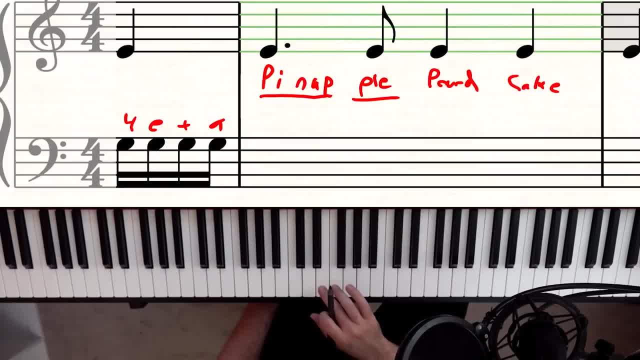 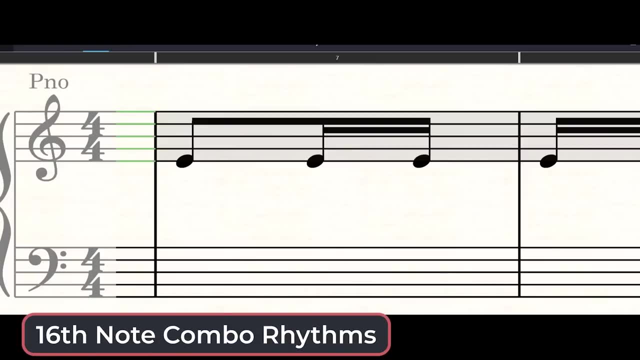 holding the dotted quarter for pine app and then moving on, pull So pineapple pound cake One and two, and three, four, Just like that. Next we gotta talk about 16th note combo rhythms. Okay, 16th note combo rhythms. 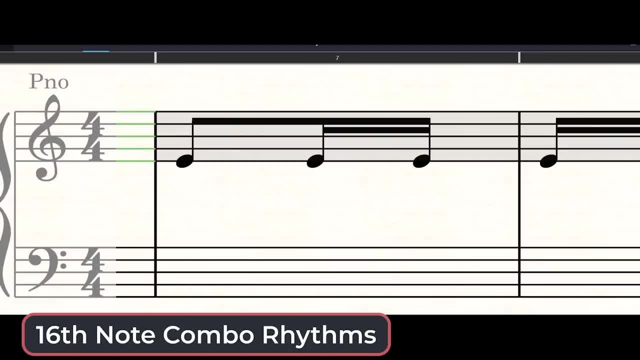 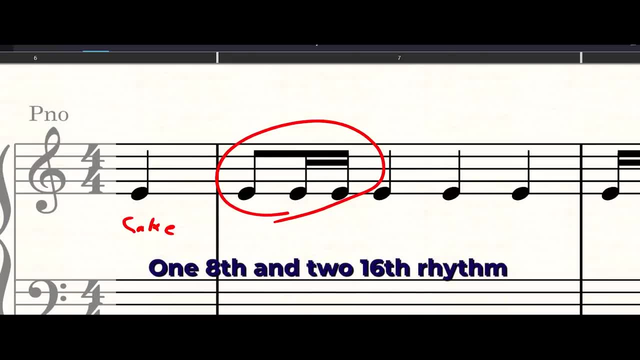 is when you're basically having mixes of eighth notes and 16th notes, And there's quite a few you need to be aware of. So here's our first rhythm, The eighth to 16th rhythm. It looks like that. Now, this one's a lot simpler than it looks. 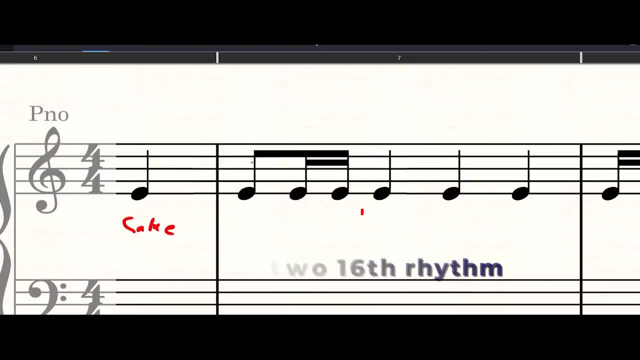 We're still using one e and a two e and a type of thing. So here's our eighth note. This is where the confusing part is, cause these are like kind of combined together Which, by the way I said before, if these are all flagged together, 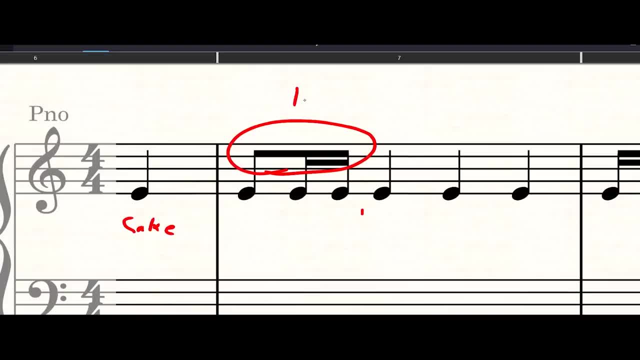 and they're all like connected. that equals one beat. So here we have one e and a. Remembering that when you're subdividing by 16th notes and you have an eighth note, it's actually gonna take up two of those. 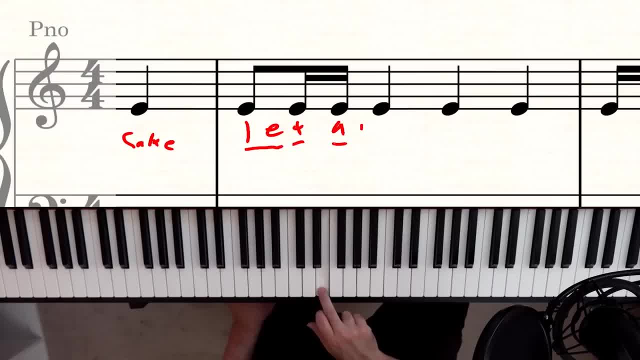 And then you'll move on and and a. So it's gonna go one e and a, And then, of course, the rest of the rhythm would be two e and a, three e and a, four e and a. But once again, it's one e and a. 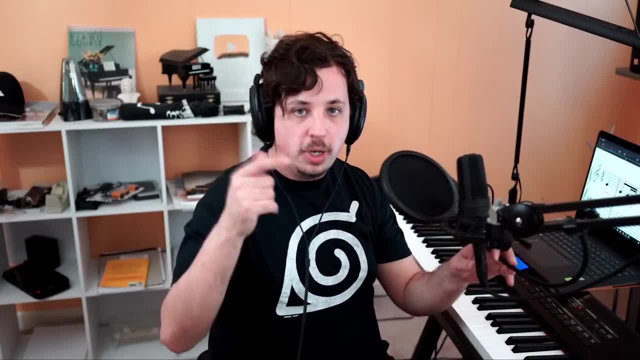 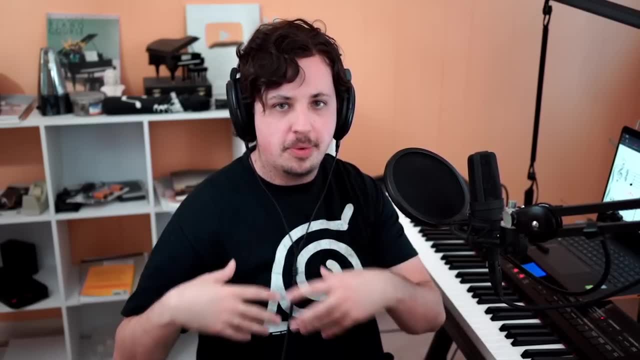 I always like to internalize these rhythms too. Instead of just going one, e and a, I like go bah, bah, bah, bah, bah, bah, Cause each rhythm has, like, a certain type of galloping to it or a certain type of cadence to it. 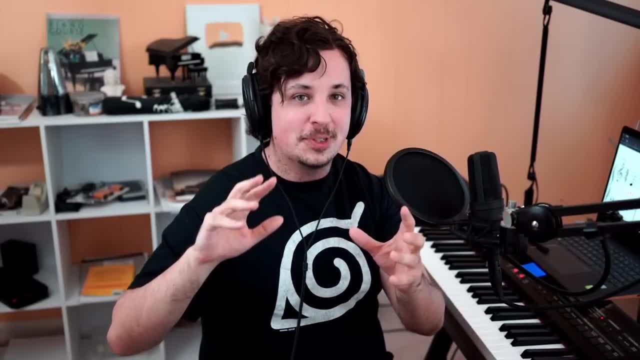 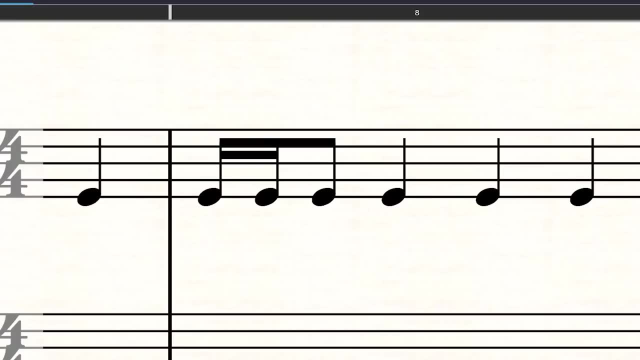 So not only just try to count them or use maybe your pineapples to count them, but also be internalizing the rhythms as well. Next rhythm: we have just building on that. Now we have two 16ths and an eighth there. 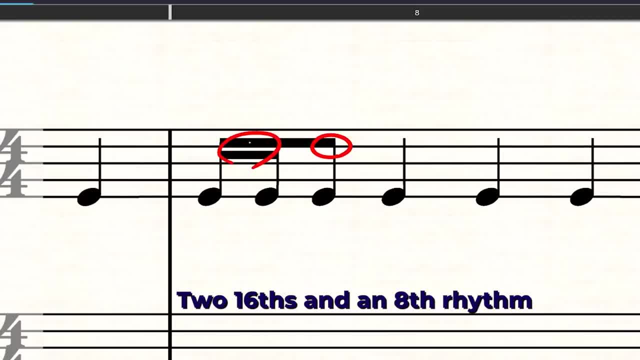 We can tell it's 16ths, cause they're double barred, And then you got one bar there, but all together they equal. what One beat? at least hopefully you said that. So now we know that we're using the one e and a. 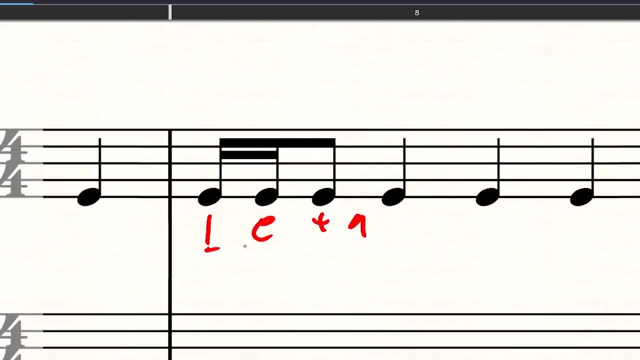 one e and a type of thing. So we have two 16th notes, one e and then and a. It's the opposite The other one. we did one e and a. This is one e and a, Or, to internalize it, bum, bum, bum, bum, bum, bum. 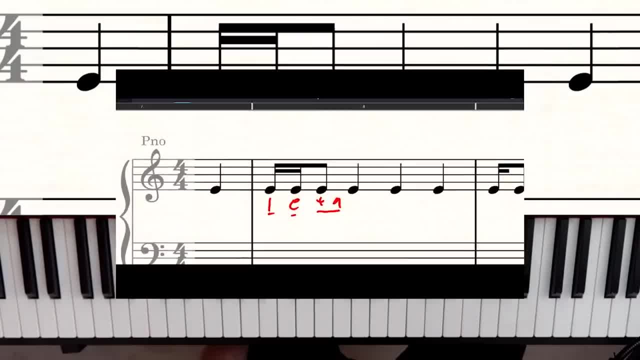 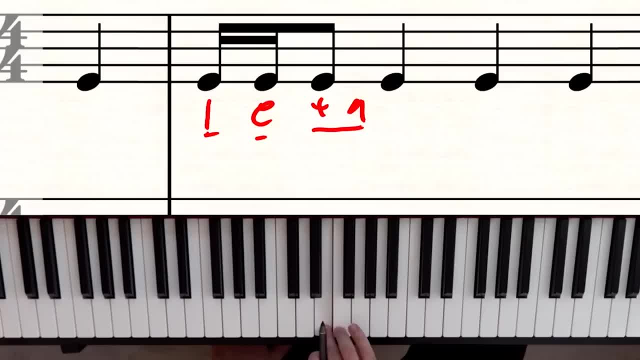 Little bit simpler there. So, of course, to play out this whole rhythm, this would sound something like this: One e and a, two e and a, three e and a four e and a, And because I was subdividing by 16ths the entire time, 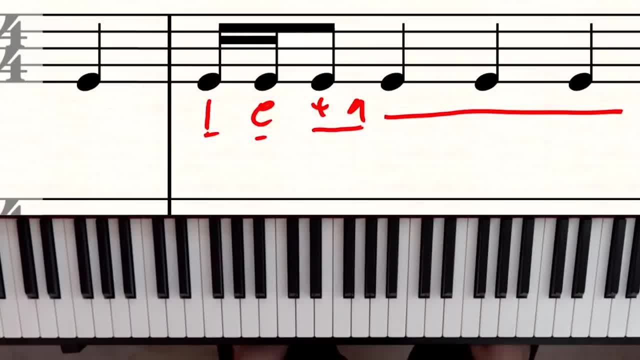 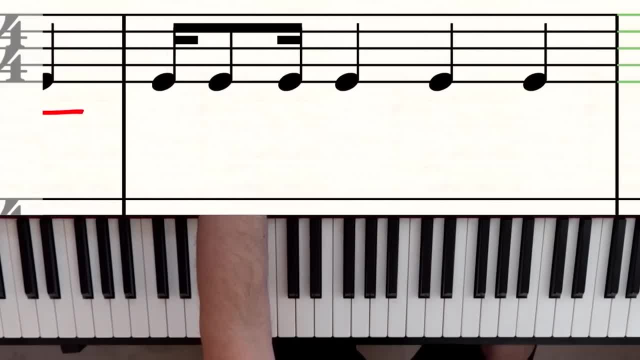 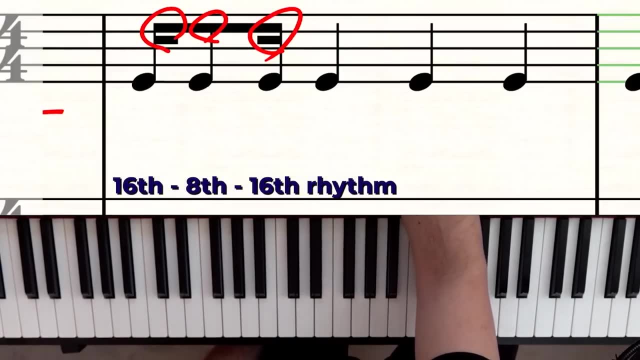 playing these the right amount, even though they're slower than the other notes, was no problem, Whereas if I would have not subdivided, I would have had to just kind of guess: Okay, we have a new rhythm here. Eighth, or sorry, 16th, eighth, 16th. 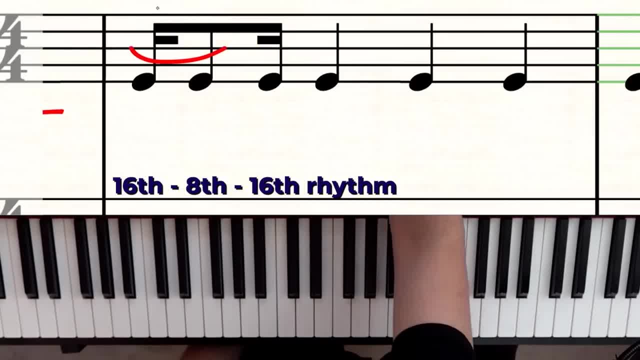 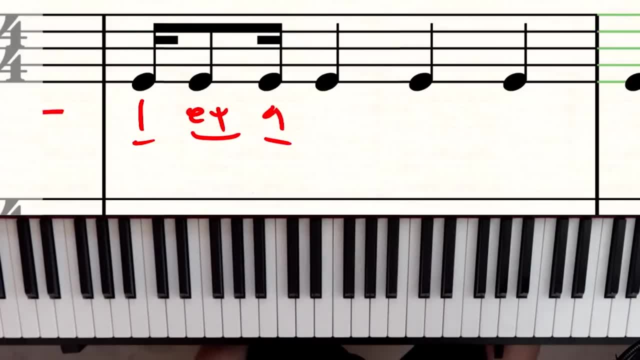 You can tell by how many flags are on each one, but all together they equal what One beat. So of course we're using our one, e and a's now. So on beat one is our 16th note. We're moving right on to our 16th note. 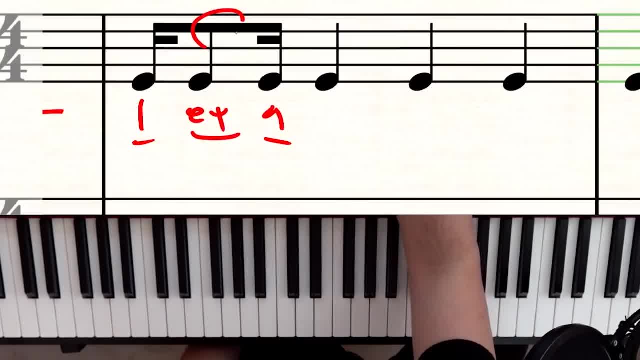 We're moving right on to e, and Keep in mind that the eighth note now takes up two of those syllables, because each syllable is worth a quarter of a beat. Two quarters equal a half, And then you're gonna move on a. 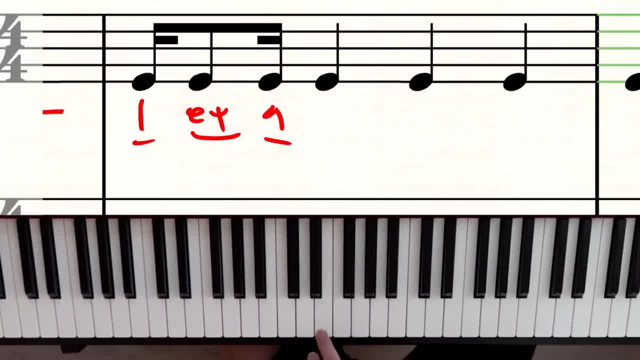 So it's gonna look something like this: One e and a, one e and a, Just playing that over and over again, Or, to internalize it: bum, buh, buh, bum, buh, bum, bum buh. 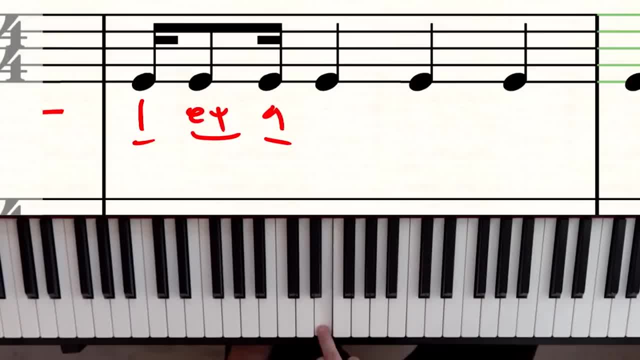 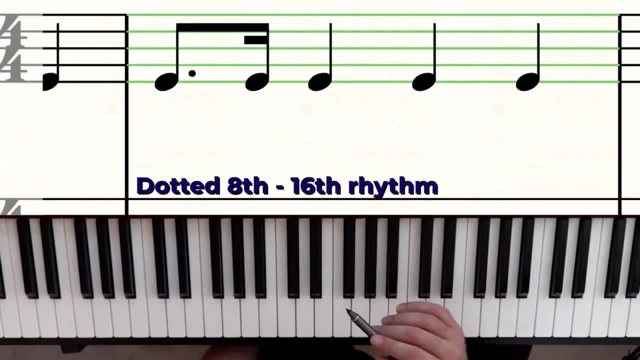 Now playing out the whole rhythm: One e and a, one e and a, Two e and a, three e and a, four e and a. On to the next one, the dotted eighth, 16th. This is the last combo pattern, at least with 16ths. 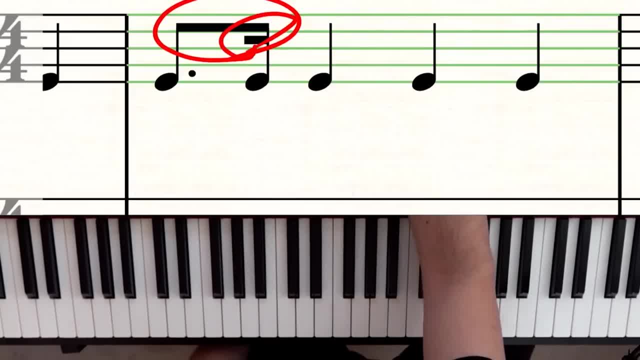 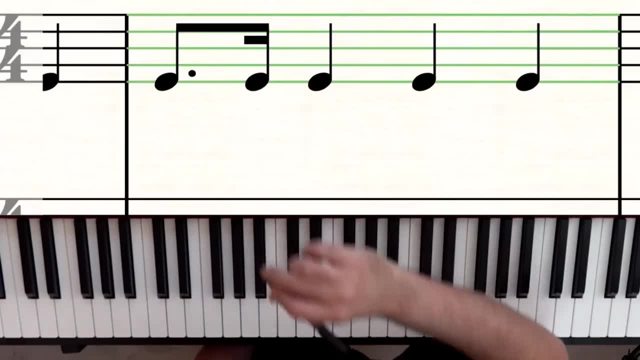 So we have our 16th here, the double flag, And then we have an eighth note here, but it's got a dot on it. So dotted eighth note, And I'm sure that looks spectacular. There we go, And then to get it together, they equal what. 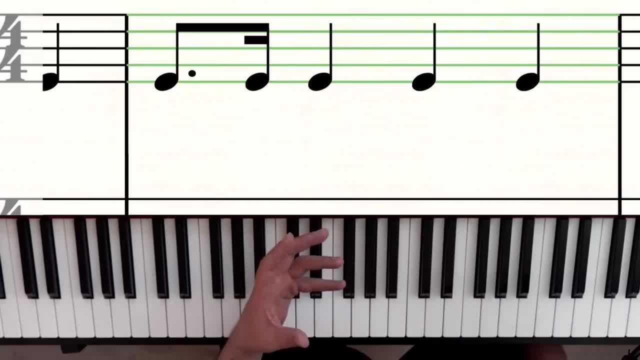 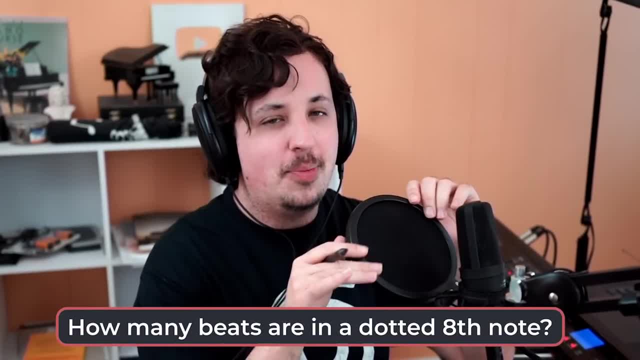 Two beats, No one beat. So now we need to talk about how many beats are in a dotted eighth note rather than a dot. Remember, dotted quarter note got one and a half. So how many does a dotted eighth get? So if you don't know, like 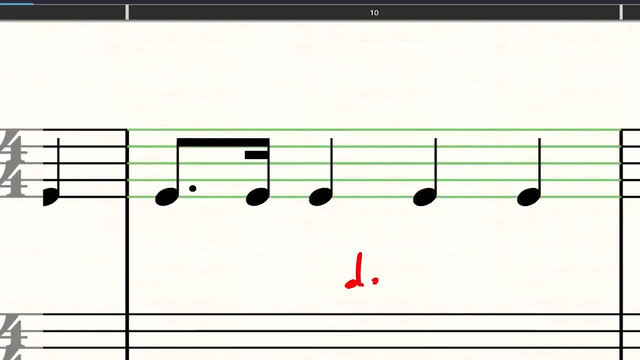 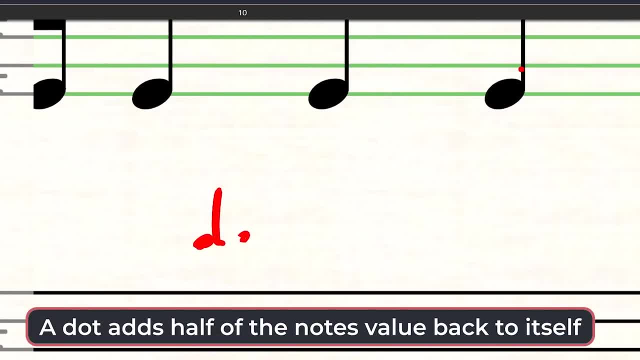 say we just I'm gonna draw like a little example down here. So if you don't know the dots, the dot will add half of the notes value back to itself. So the reason a dotted quarter note gets one and a half beats is because it's one plus a half of one. 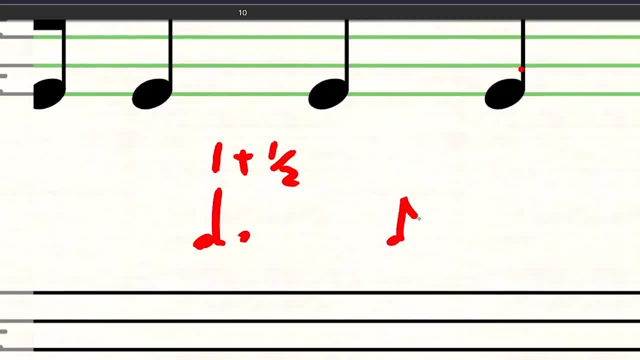 which is one and a half. So what about a dotted eighth note? Well, an eighth note gets half of a beat, right, And what's half of one half a quarter? and then you have to use your math from school plus one fourth, make them the same. 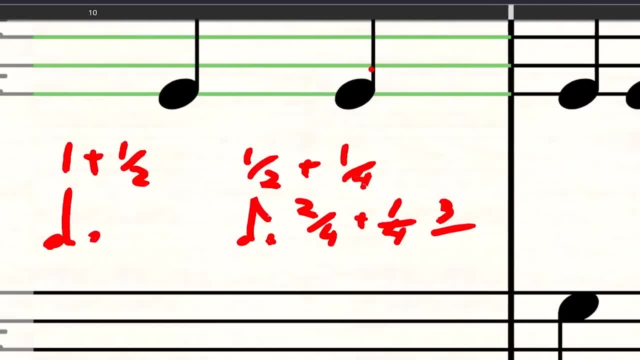 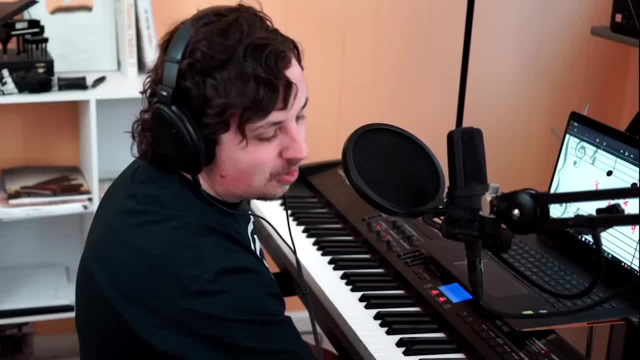 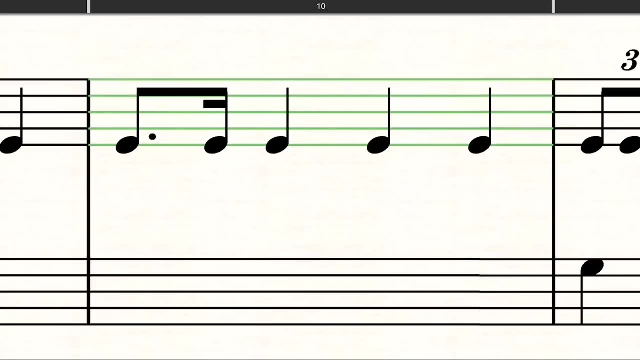 So a dotted eighth note- I'm sure this is the math you wanted to see today- is three quarters of a beat. So how in the world are we gonna count three quarters of a beat? It's actually really easy Using subdivision. So remember earlier when I was talking about 16th notes. 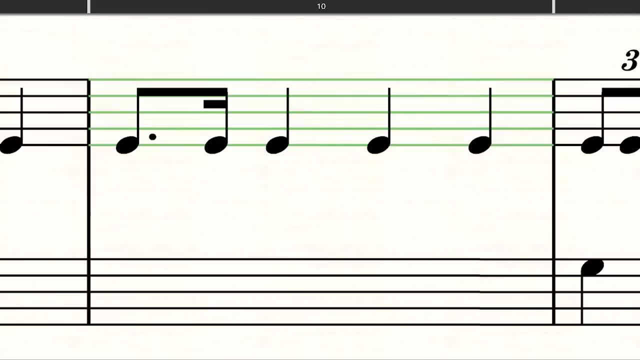 one E and a, two E and a, that each of those syllables equaled a quarter of a beat, and we need this thing right here to equal three quarters. So it's very simple really. It's just gonna take up one E and. 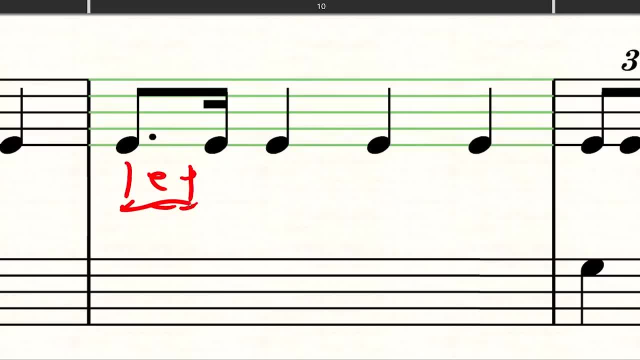 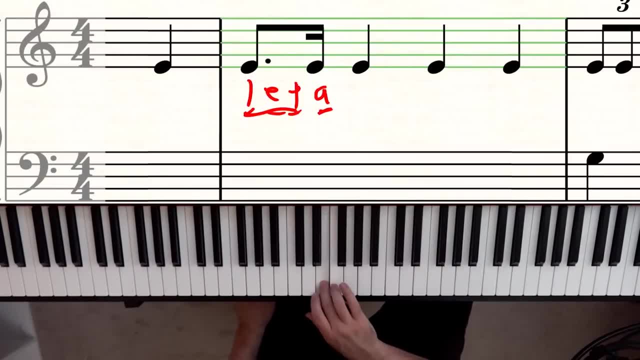 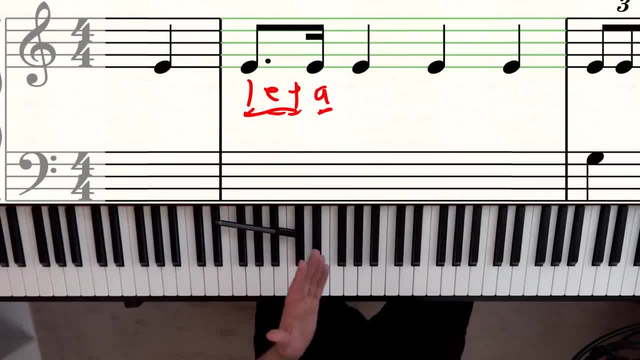 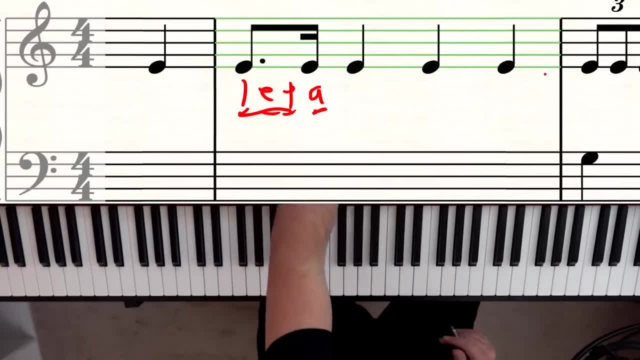 Four, E and a, Or, to internalize it, bah bah, bah, bah bah. it has a certain type of cadence to it, like the others, So you also want to try to internalize it. And moving right on to triplets, 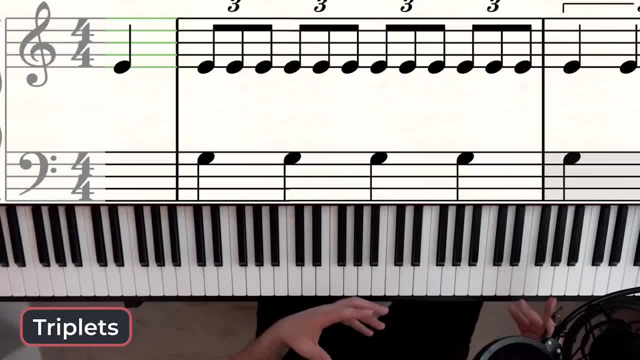 this is where things get interesting. So now we're not dividing into twos or fours, we are dividing into threes, And a lot of people struggle with this, especially moving from threes to twos, And I have a little trick here for you. 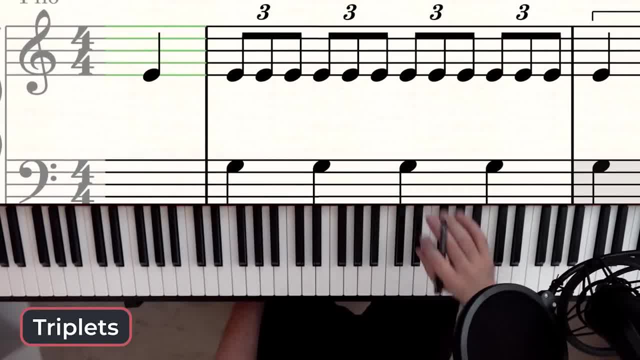 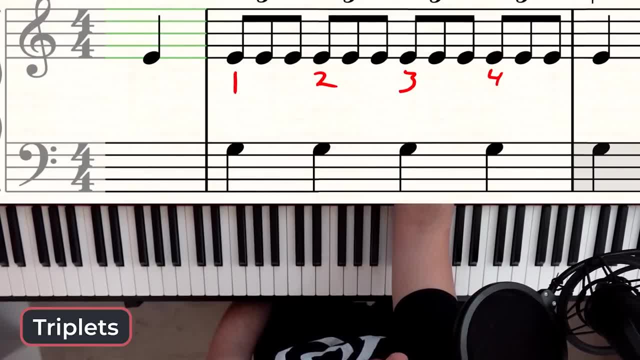 to get used to that. So let's talk about triplets for a second. So now we're splitting each beat into thirds, and this is how we do it. So let's just write out our three or four beats here. rather, We can't count today. 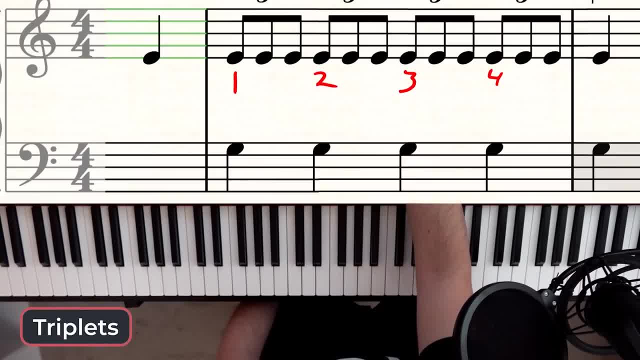 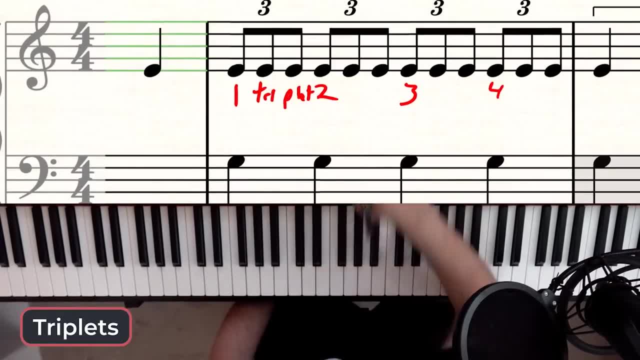 And this time we're not using ''and'' at all, because that won't work. That's only for counting into two equal parts. So I use one triplet, one triplet, two triplet, three triplet, four triplet, and then I'm just gonna play quarter notes in the left hand. 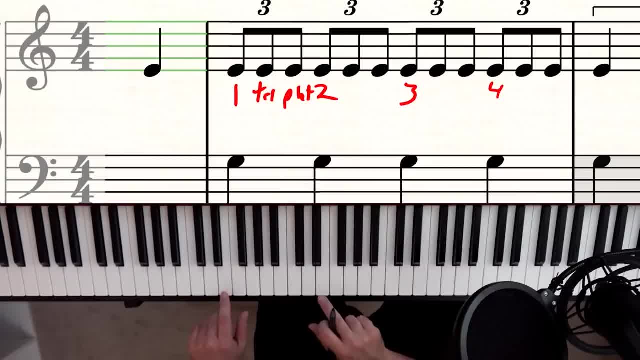 One triplet, triplet, two triplet, three triplet, four triplet, rather than one and two. and it's one triplet, two triplet, So a little bit faster, but three even parts. So here I have an alternating rhythm between a triplet, an eighth note. 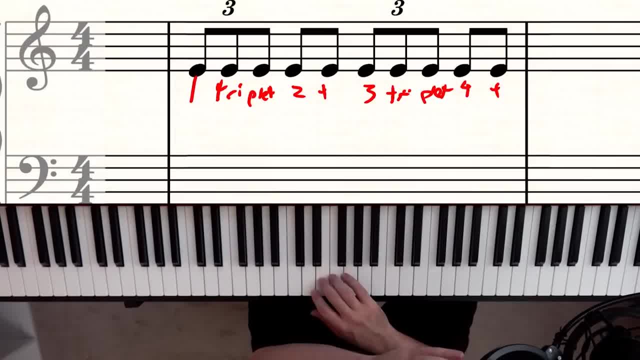 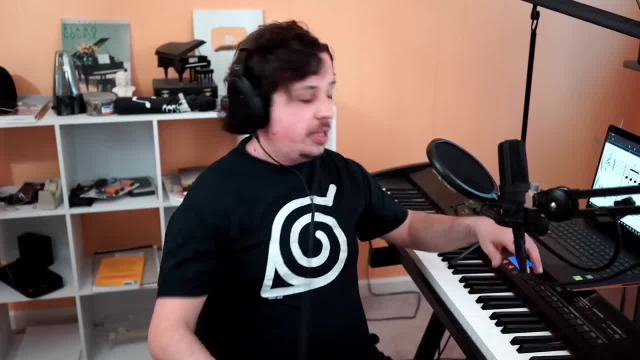 a triplet and an eighth note. So quite simply this would be counted as one triplet two and three triplet four, and. But a lot of students ask me all the time, Tim, I really have trouble moving from triplets. 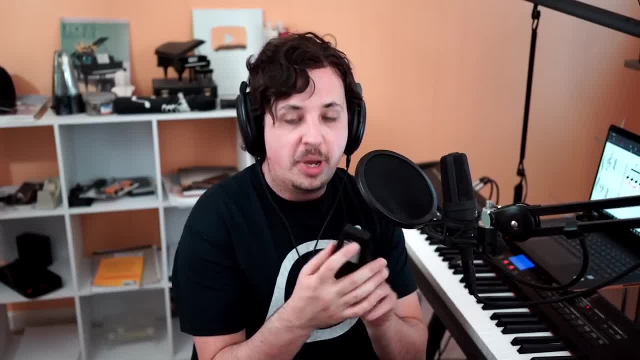 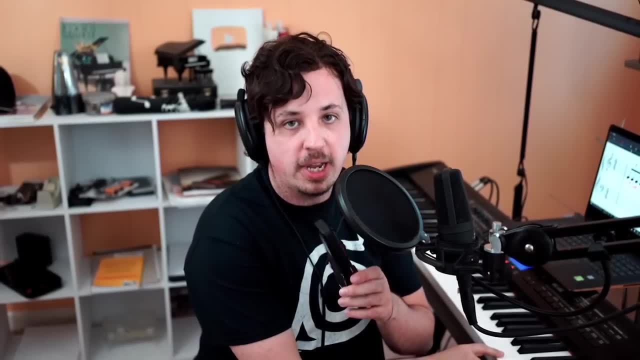 eighth notes and back forth. So you're gonna have to use our best friend ever, the metronome. set it to four, four, one, two, three, four And then, in time with the metronome, see if you start out with eighth notes, right. 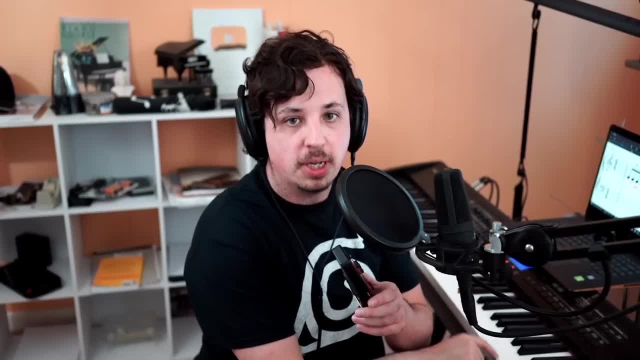 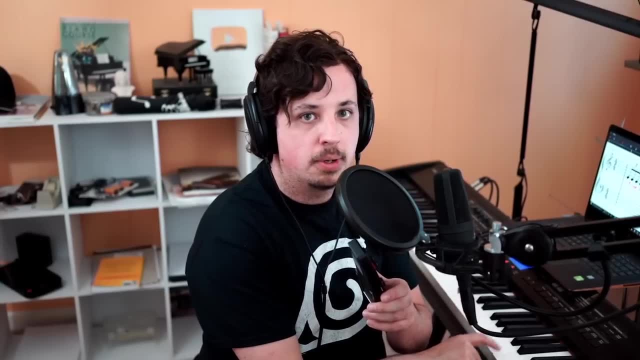 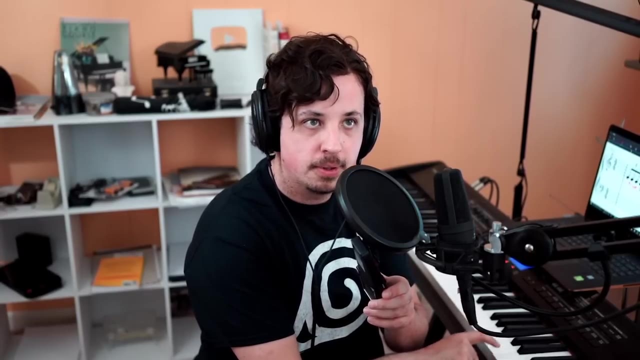 Two, three, four. so we go one and two and three and four. Now, when you get used to that, try triplets, So move back and forth between those two, And then what I want you to do is then we're gonna make it real interesting. 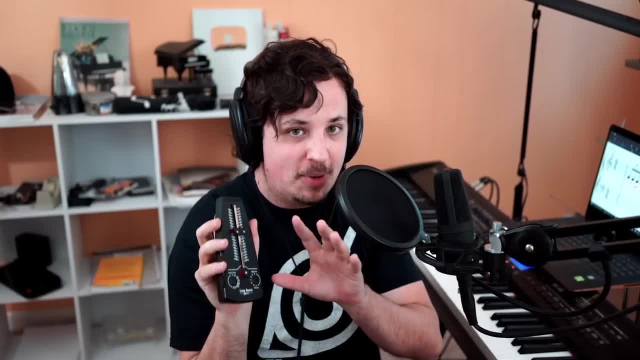 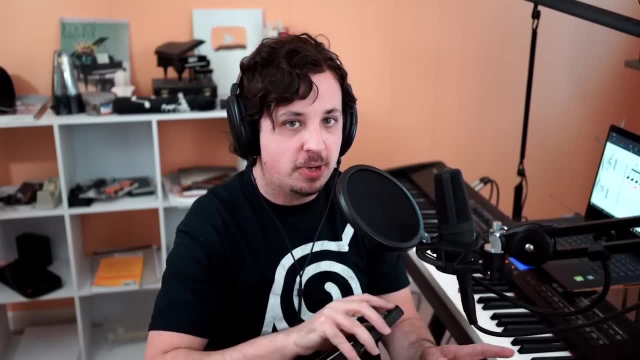 You're gonna play one beat triplet, the next beat- eighth notes, the next beat triplet, the next beat eighth notes. It's just like the rhythm I gave you on the sheet right here, So let's see if we can do that together. 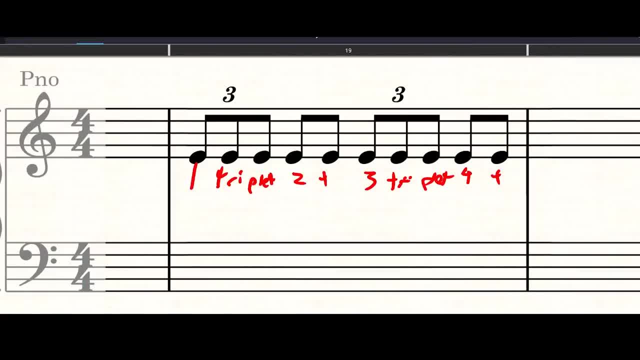 So here's our four beats. I always recommend you just kind of like a little bit faster, So let's see if we can do that together. So here's our four beats. I always recommend you just kind of like little bit faster. 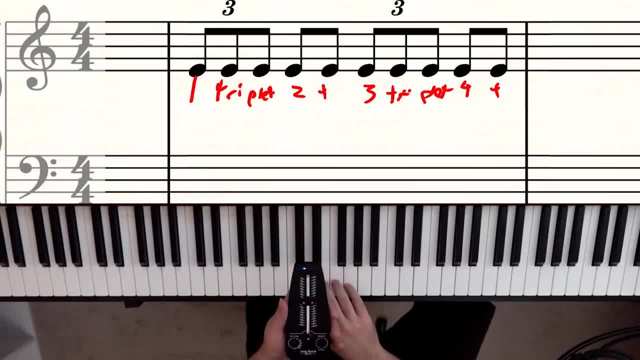 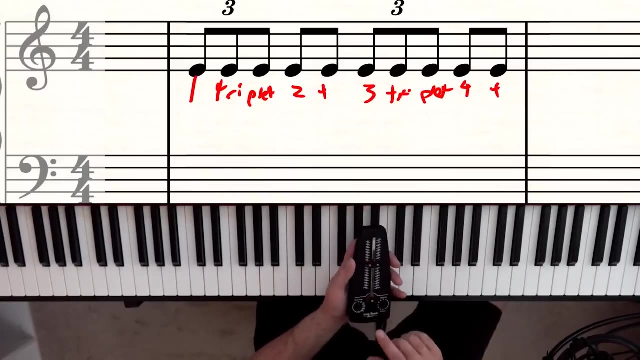 So let's give it a play for a minute to internalize the rhythm: One triplet, two and three triplet four and one triplet two and three triplet four and one triplet. So as you can see, with the metronome we were moving from triplets to eighth notes. 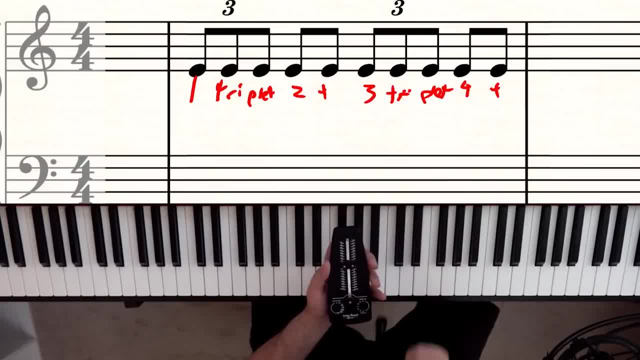 and the metronome was actually keeping each of those beats for us, So I could shift between triplets and eighth notes, triplets and eighth notes, And using the metronome, I could also hear when I was getting a little bit off. 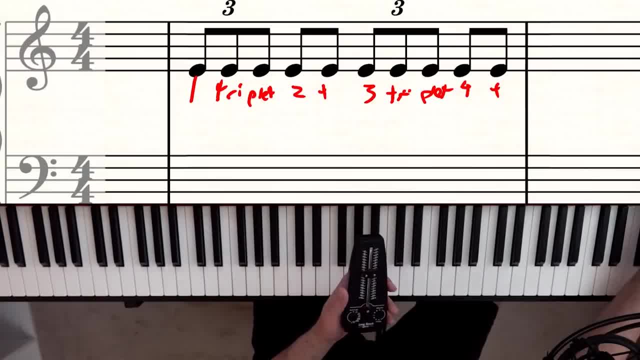 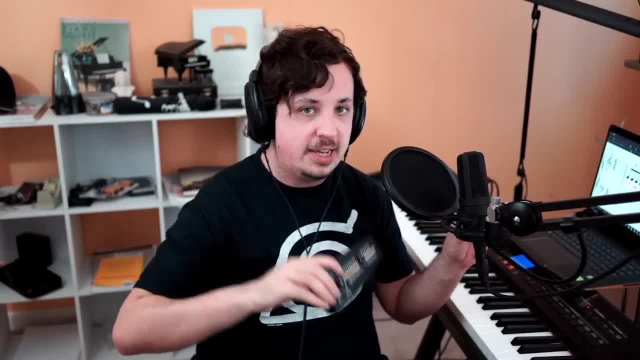 and then I could go back and make it more solid. So what I recommend you do at home is actually just to use the metronome and do what we did just now, Alternating between triplets- eighth notes, triplets, eighth notes. 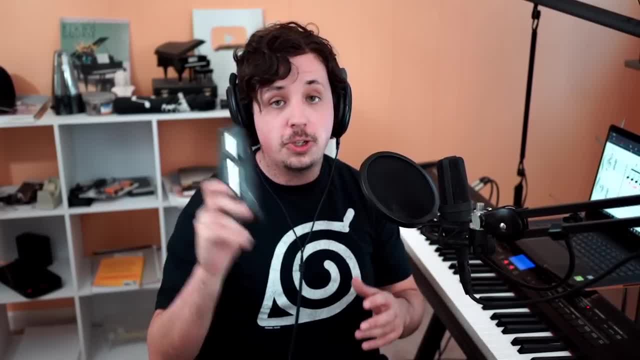 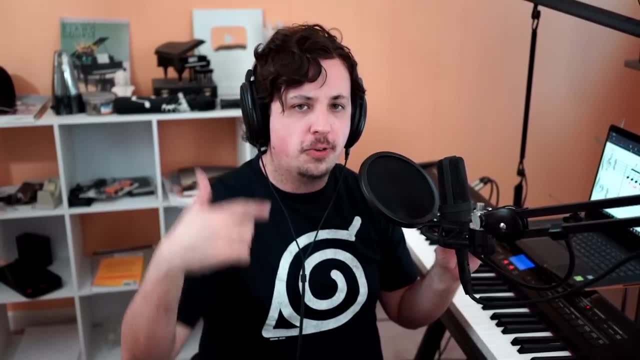 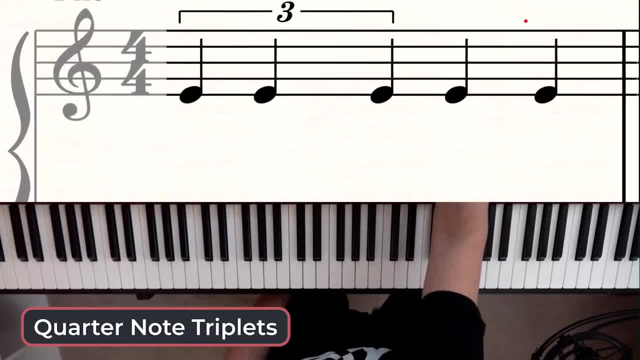 So that you can remember it a lot easier. Now, if you're extremely unlucky, you've seen quarter note triplets, So how in the world do you count these? I'm gonna be honest, you're not gonna see these in your music a lot. 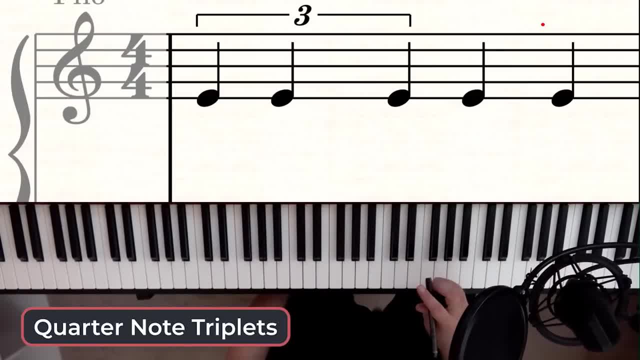 but there is a chance you'll see them, So let's do this. So we now have three quarter notes underneath our triplet, which is a quarter note triplet, And the question is is how many beats is this going to take up? Well, I wanna give you a little hint. 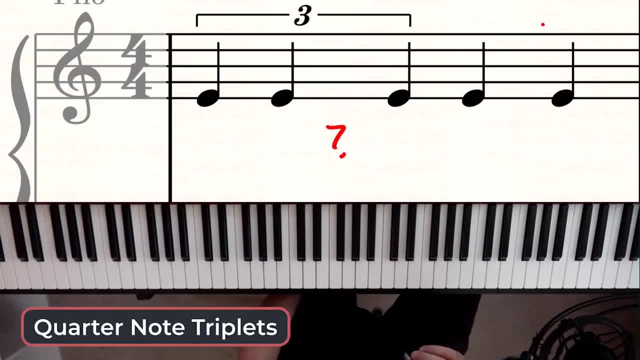 The amount of value that a triplet takes up is always like double. whatever the note value is is underneath it. So if these are quarter notes, you're not adding them together. If that's a quarter note, the total amount of beats that all three of those. 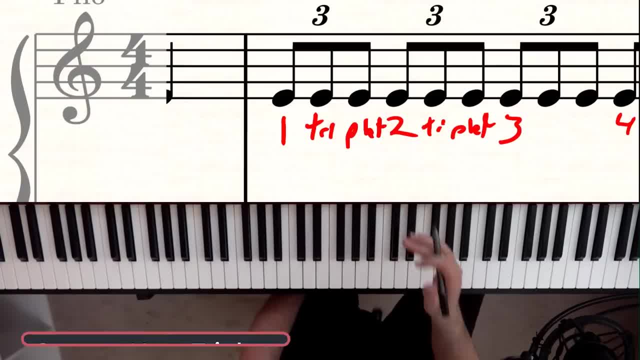 are gonna take up together is a half note, Just like with the eighth note triplets. that they were three eighth notes put together, not really, but in this case, but they really took up the value of the next note up, which was the quarter note. 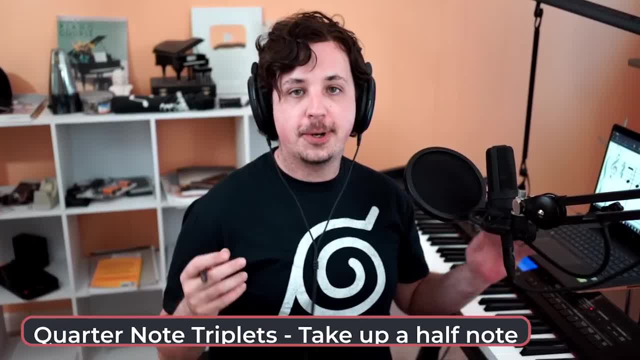 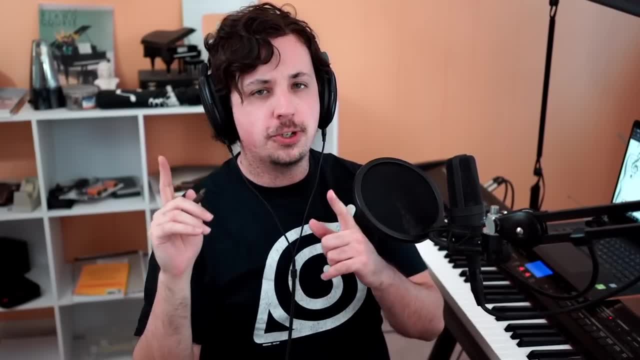 So if you have quarter note triplets it takes up a half note. So to count this, we're going to be counting actually two beats of one triplet, two triplet. We're using the same thing but it works just slightly different. 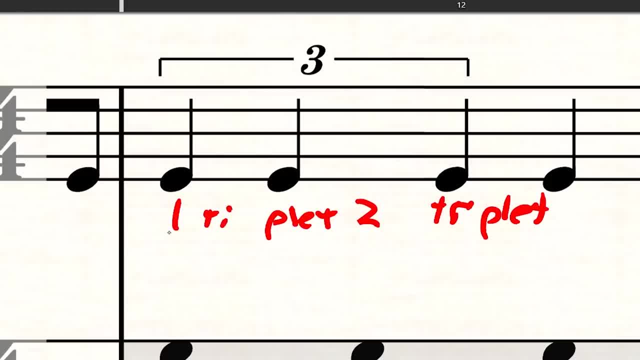 So we're counting out one triplet, two triplet, except instead of each of the notes in the triplet just taking up one syllable, they're gonna take up two syllables. So this gets a little tricky, but you will get the hang of it. 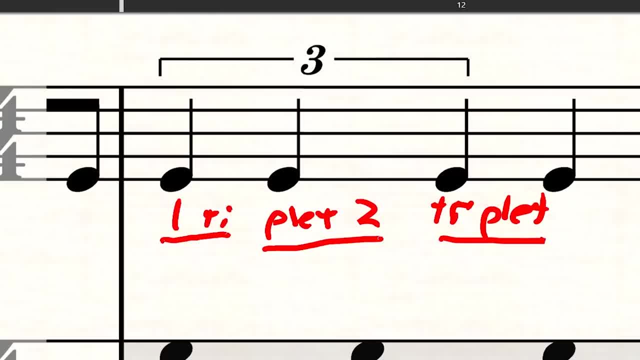 So instead of one triplet, two triplet, it's one triplet, two triplet. I know it sounds a little bit off putting, but you'll get used to it. One triplet, two triplet, one triplet, two triplet. Let me show you on the piano. hold on. 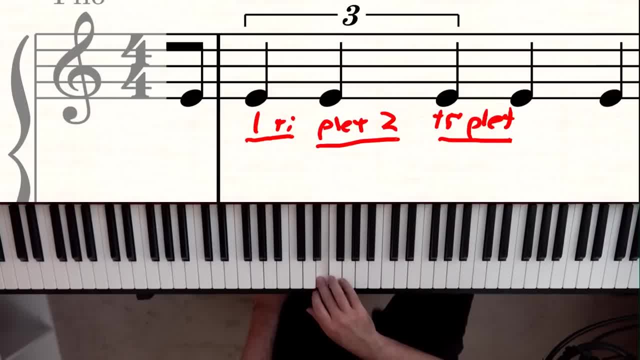 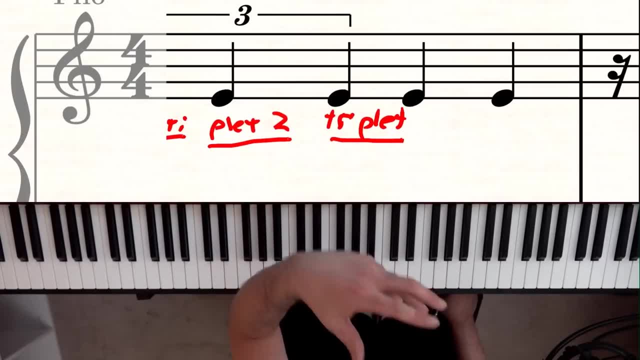 One triplet, two triplet and then three and four, and Probably use a metronome to make sure I'm getting into the quarters a little bit, but that's how you do it. You just say one, you would do two beats of triplets. 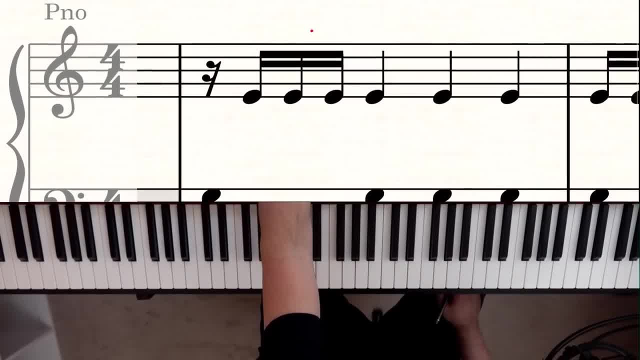 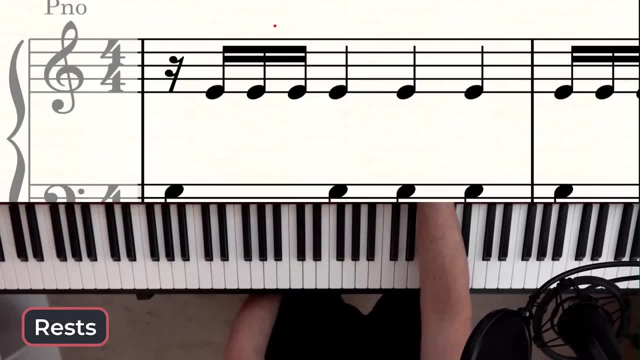 but just two syllables on each one. Now I got another kind of combo rhythm, combo rhythm for you right now. This is the 16th rest, 16th notes. This is very easy to count because the 16th rest just gets. 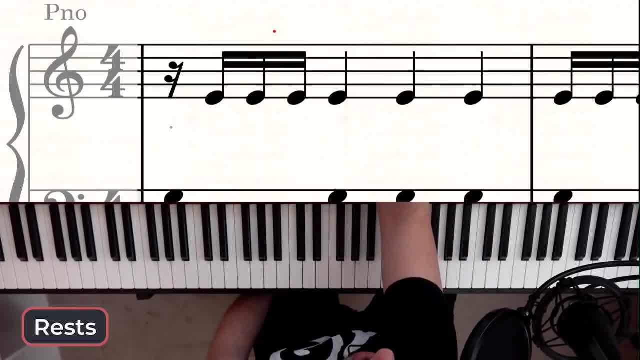 one quarter of a beat, like a 16th note does. So we're still using our one E and a, except we're not playing on beat one. So it'll go one E and a, one E and a, two E and a, three E and a, four E and a. 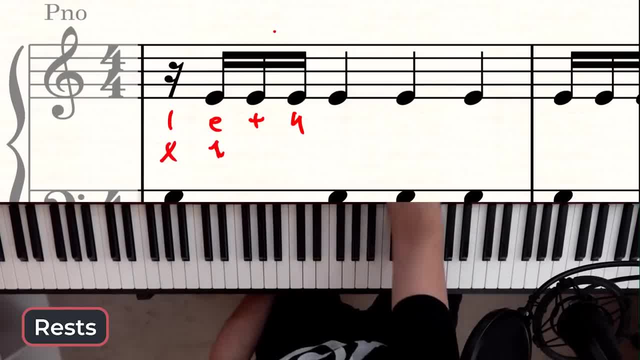 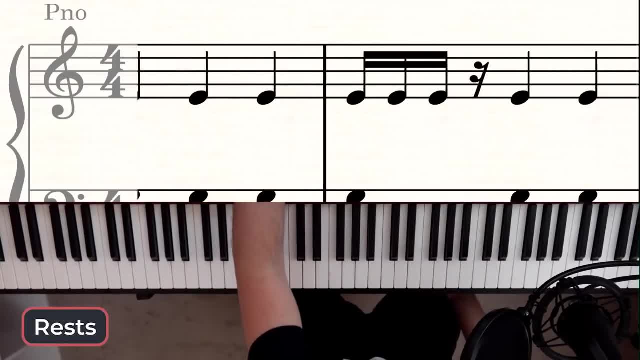 one E and a. So you wanna kind of plan your attack on E instead of that beat. So you would like kind of tap your foot and then move onto the next note. That one's a little bit simpler. The opposite of that is three: 16ths, 16ths, 16ths, 16ths. 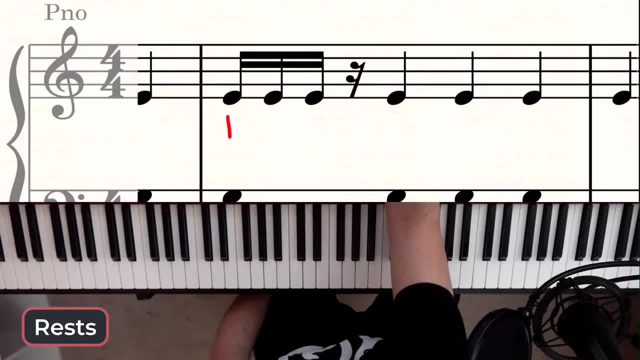 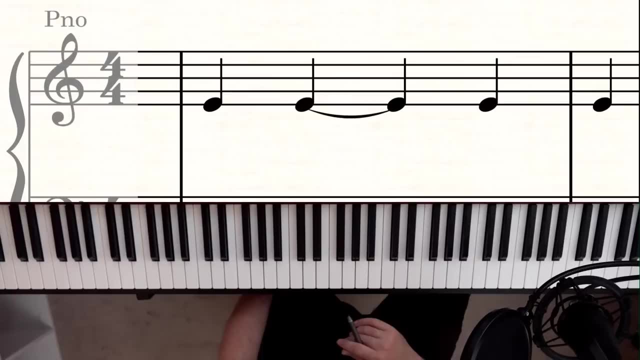 16th rest. So you would go one E and and then a nothing. So one E and one E and a, two E and a, Playing out the whole rhythm: one E and a, two E and a, three E and a, four E and a. 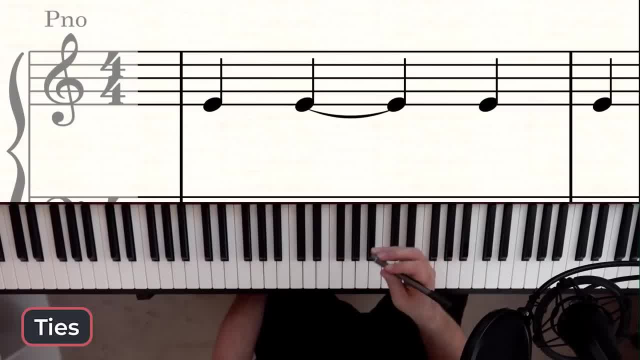 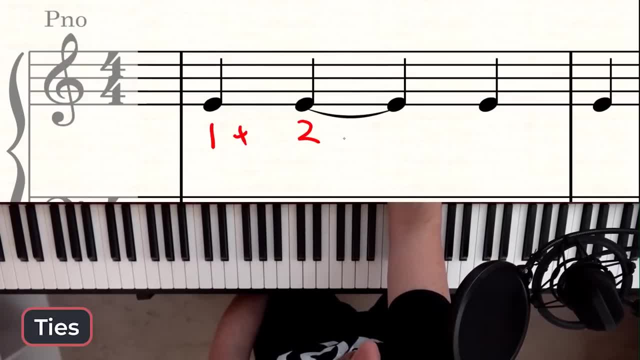 Next we have ties, Another one a lot of students ask me about. So we have four quarter notes here, very simple, but we should probably still subdivide into eighth notes. Why do you think that is? Well, that's so we can count more accurately. 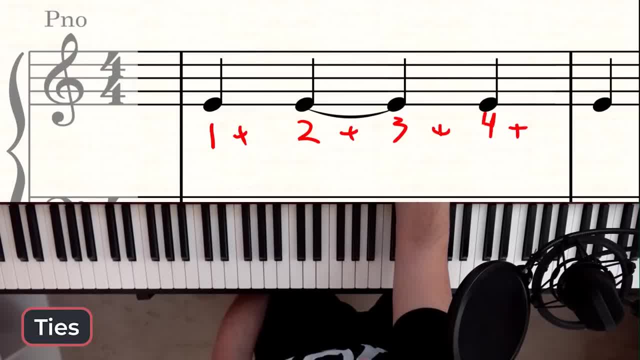 because the longer you hold notes over, the more guess time that your brain has to do. So this is very simple. Normally this would be counted as one and two, and three and four, and, but this time we have a tie. A tie ties over beats. 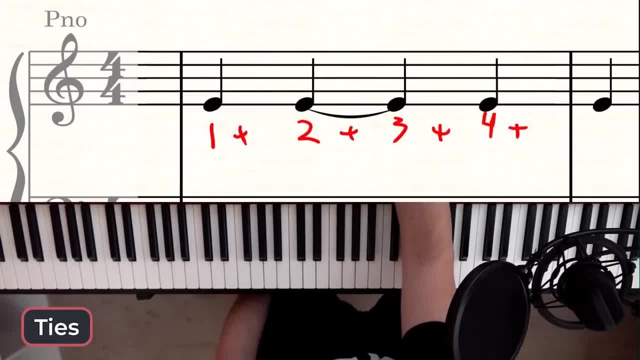 So this quarter note here, tied to the other quarter note, isn't just gonna take up two and it's gonna take up three and two. It's almost like a half note. Now you may be asking why wouldn't you put a half note there? 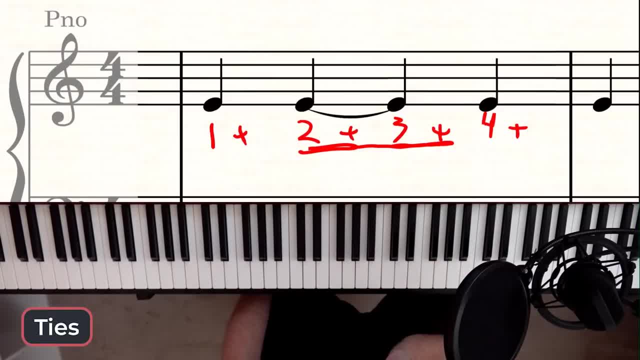 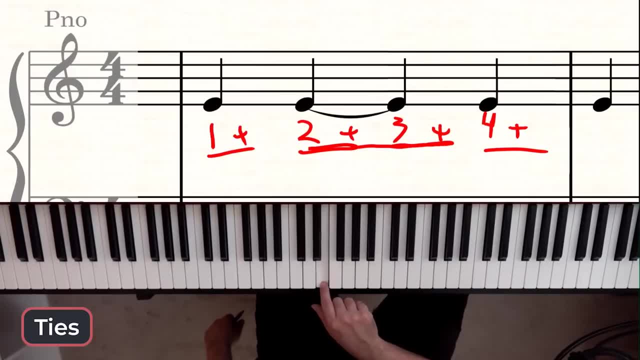 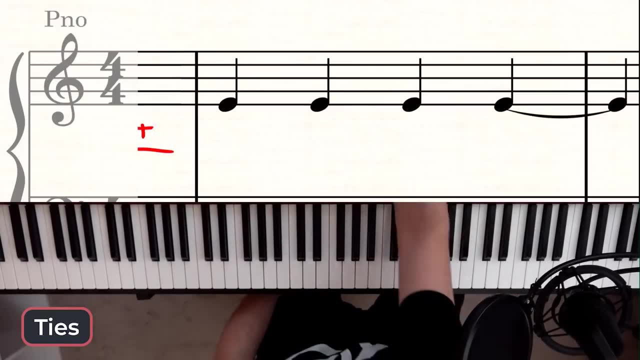 That's a very good question. Well, there are other uses for ties, as we'll find out in a minute, but this is how we'll play this rhythm. So it's gonna go one and two, and three and four, and Now here's where ties really come into play. 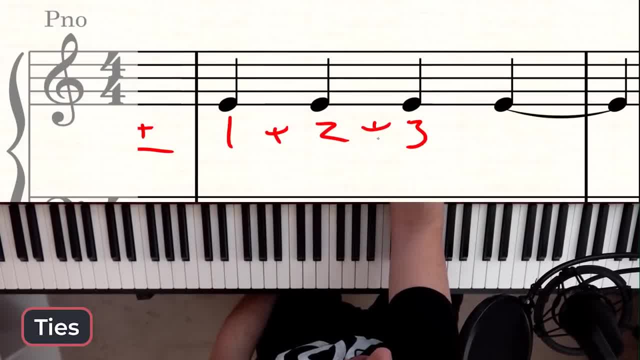 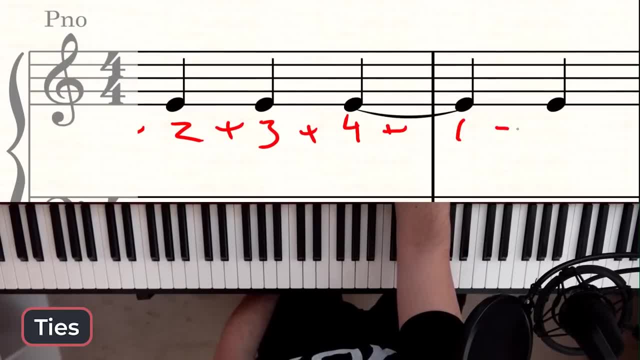 So here we have beats one, two, three- I guess we'll just put ands in there, why not Four? And? and now we're tying beat four or four and rather over with one, and So these will all be tied together into a single beat. 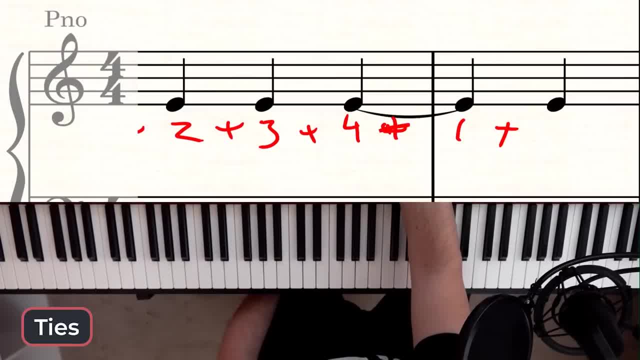 or into a single hold over, rather. So this is why you would need a tie right in an instance, because you can't draw a half note. It won't, it seriously won't. let me do it. You can't draw a half note in between measures. 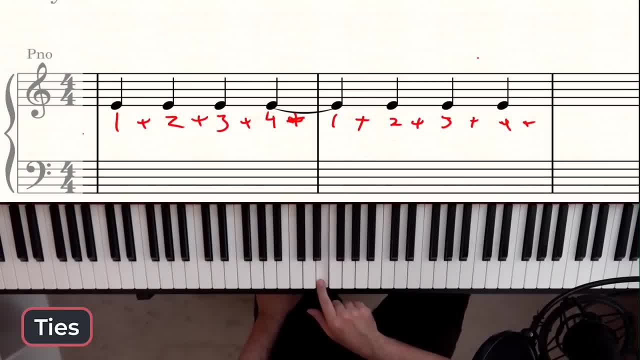 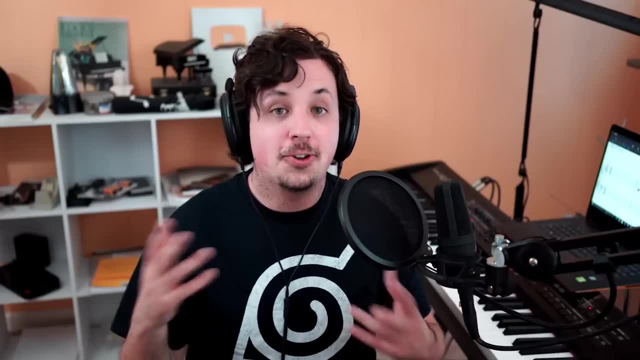 So this whole thing would just be counted as one and two and three and four and three and one and two and three and four, and Keep in mind that I held over from four and didn't press that note again for and As our ninth rhythm pattern at the end. 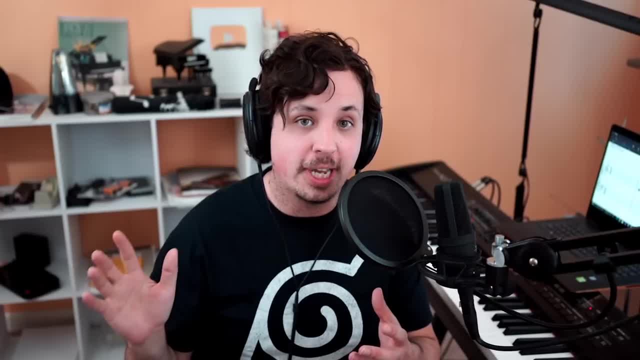 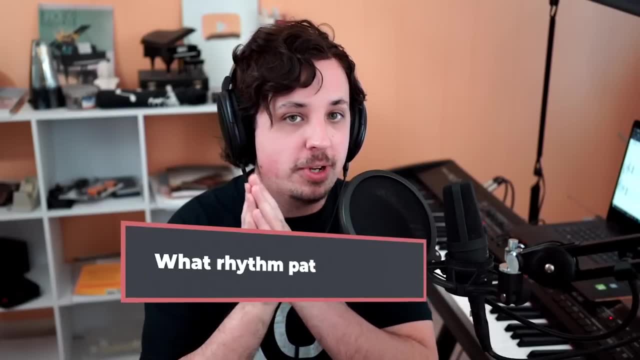 I actually have a really special tip for you. It's really really useful when counting rhythms accurately. But before that, I want you to leave a response in the comments, because I have a question for you. What rhythm patterns do you struggle with the most?